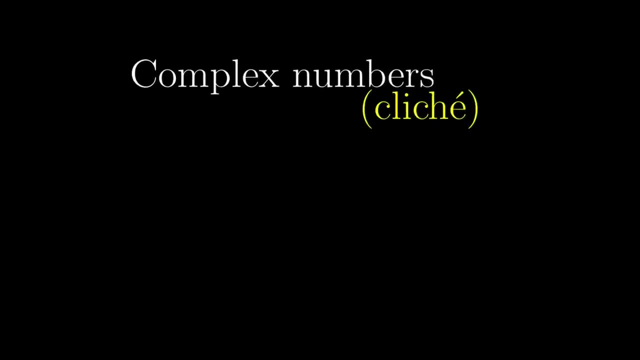 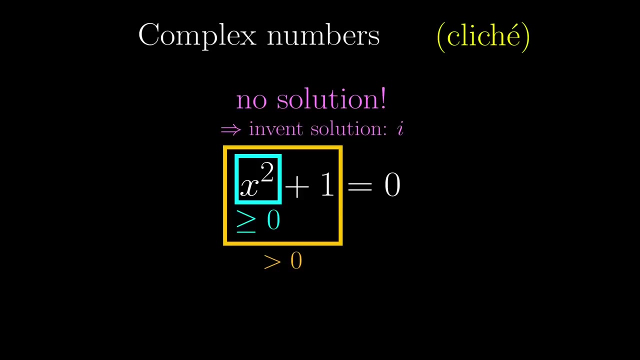 The most cliché motivation of complex numbers is to stare at this quadratic equation and say: oh look, squares are always non-negative and if we add 1 to it it is surely positive. so this equation has no solution, and that's why we invent a solution called i. But the problem 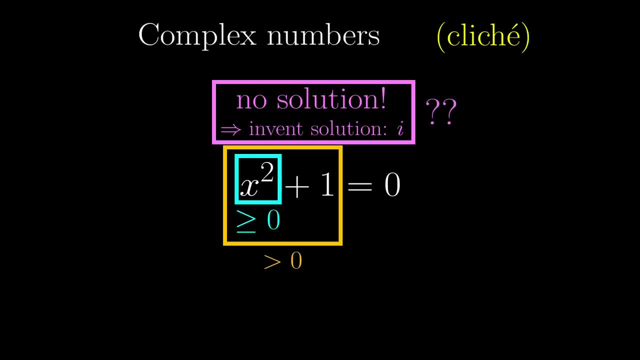 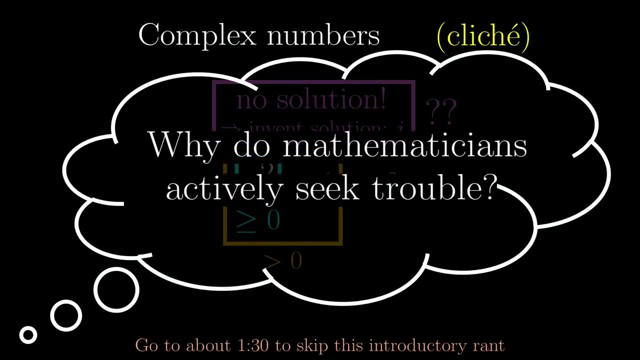 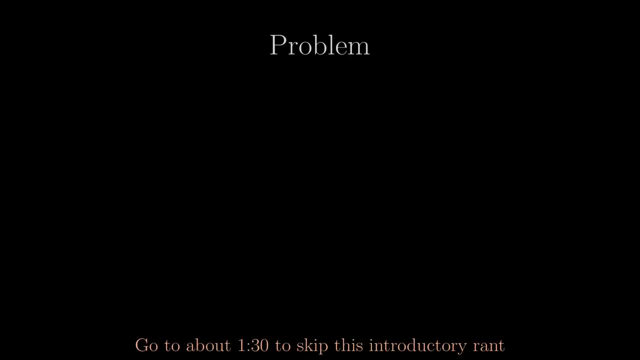 is that having no solution doesn't mean we have to invent one. If anything, it makes you think that mathematicians actively seek trouble addressing a problem that could be ignored, because having no roots is not a problem. The actual problem arises when we try to solve this. 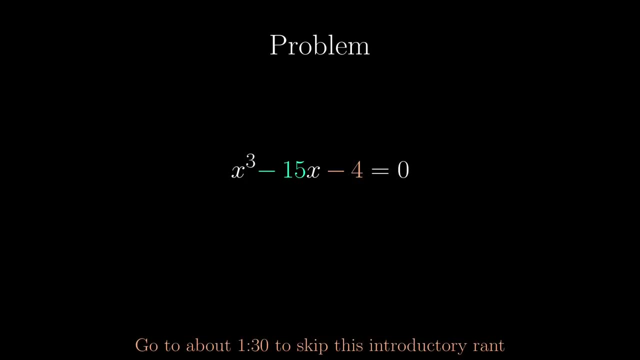 cubic equation with a general method By inspection, 4 is a totally legitimate root because its cube is 64, and multiplying by 15 gives 60, and indeed 64 minus 60 minus 4 is 0, so 4 is indeed a root. 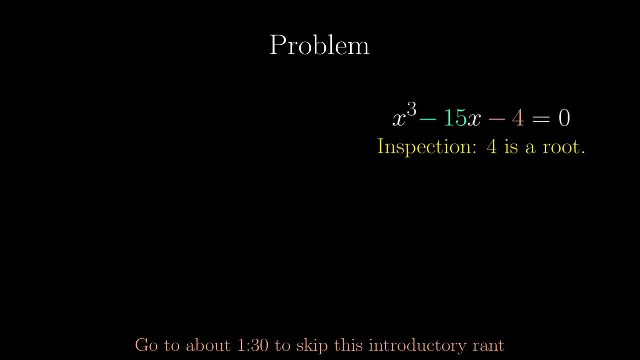 But we might want to work this out in a more systematic way than inspection. This can be done using Cardano's formula, and all we need to do is to substitute p and q, and this is what we got. So we really have to come to terms with square root of negative numbers. Not only that, 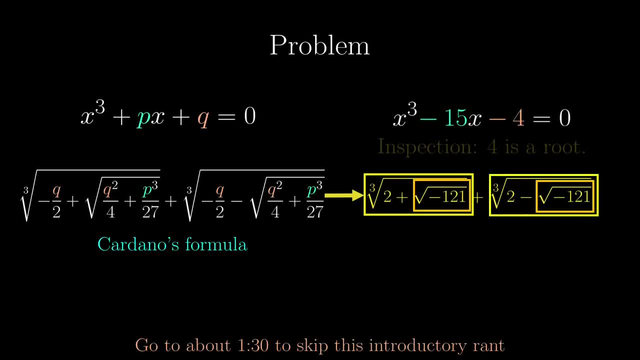 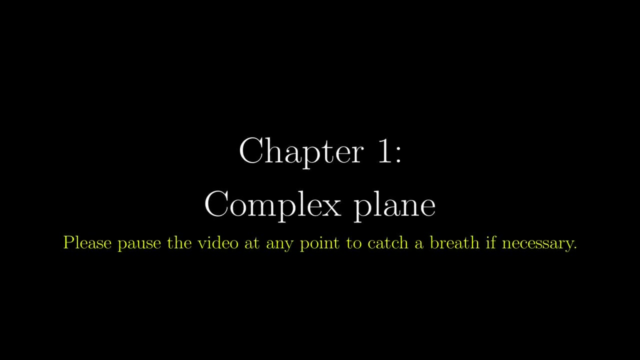 we also need to know how to take cube roots with these weird stuff. This time we can't just ignore this, because there is a root 4.. And this was really what prompted the study of complex numbers. This is one way of representing complex numbers. i here denotes the square root of negative 1,. 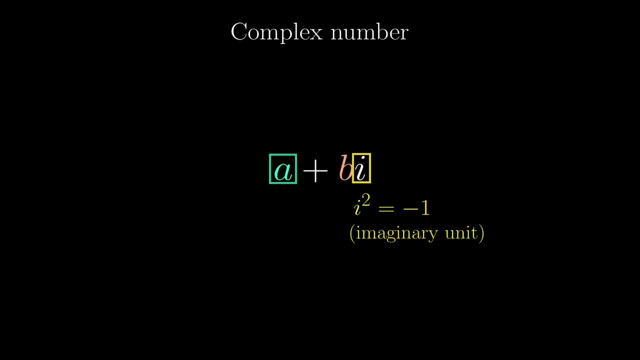 called the imaginary unit. a and b are plain old real numbers and this time a is called the real part. without the attachment of i and b is the imaginary part multiplying the imaginary unit. In other words, both real and imaginary parts are real. 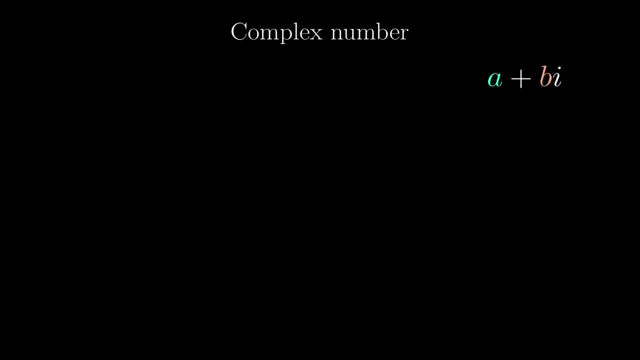 So we need two real numbers, a and b, to specify a complex number which could naturally be put on a coordinate plane. So this point having coordinates a, b corresponds to the complex number a plus b, i. Because of this correspondence we can represent all complex numbers on a plane. 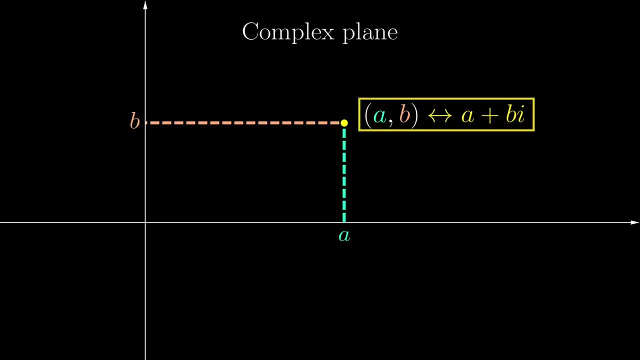 called the complex plane. We can also use a complex plane to represent all complex numbers on a plane. we usually denote a complex number as z, which is why it can also be called the z plane. Now, since a is the real part, b is the imaginary part, the horizontal axis is the real axis. 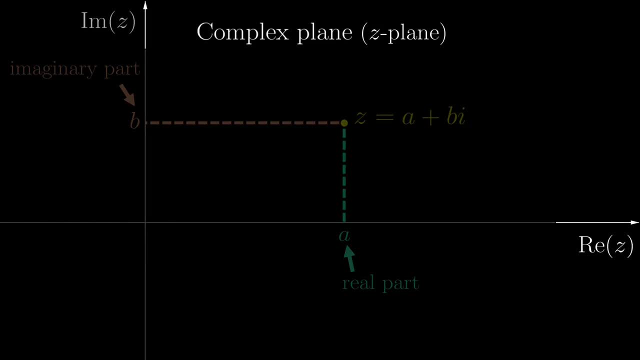 usually labelled as Re, and the vertical axis is the imaginary axis, usually labelled as Im. However, this is only one way of thinking about this point, the Cartesian way. There is another, the polar coordinates. R here specifies the distance from the origin, called the modulus. 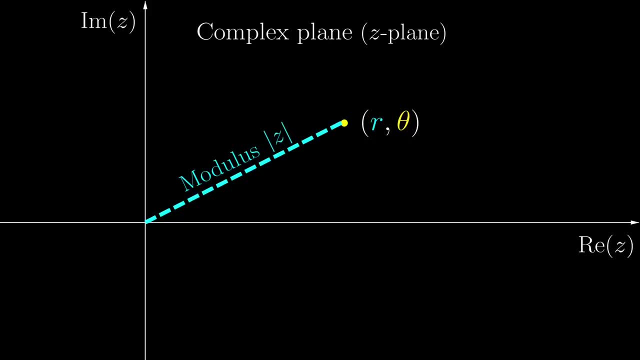 and denoted as the absolute value of z. Knowing the modulus is not enough, because those on the circle all have the same modulus, So we also need to specify the angle theta made with the horizontal, called the argument and denoted as arg. However, this can spark some arguments. 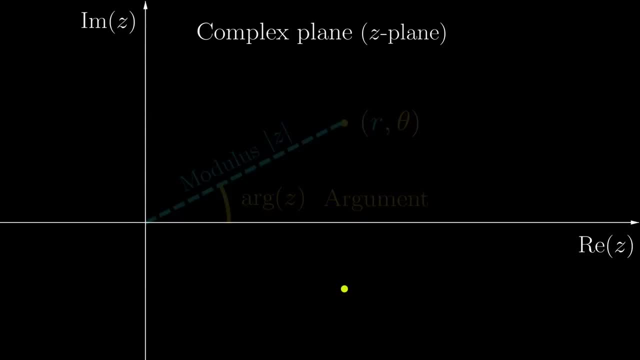 pun please. So we need to specify the angle theta made with the horizontal, called the argument and denoted as arg. However, this can spark some arguments- pun please, much intended. What if the point is down here? The modulus is perfectly fine, but for the argument. 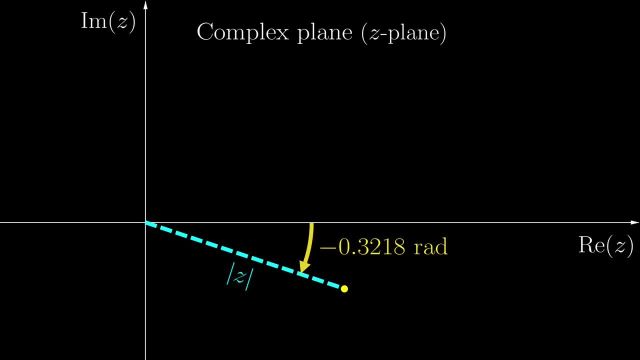 would you go clockwise, registering as a negative angle, or would you still go counterclockwise all the way around, registering as a positive angle? It really depends on your convention. I mean, technically, we can also add another 2 pi radian to it whenever we want. 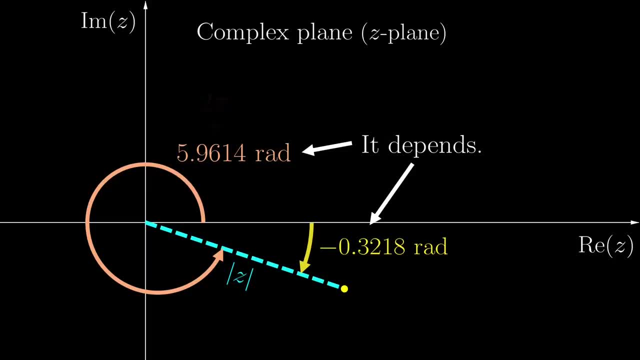 As long as you have a clear convention and stick to it, you are fine. In this case, the usual convention is to consider the negative argument. Essentially, we want the argument to be in the range negative pi, pi, so on the upper half plane. 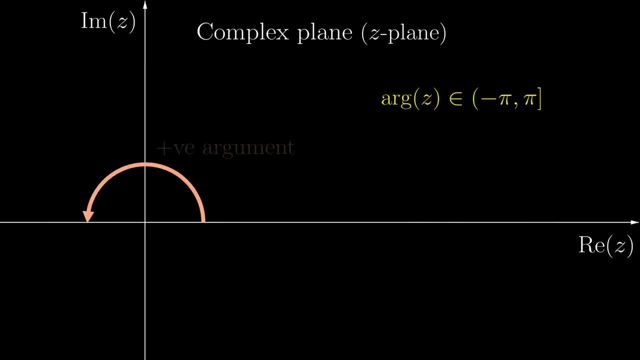 we get a positive argument and on the lower half plane we get a negative argument. The edge case is the negative real axis. In this case we say that the argument is positive. pi If we plot the argument against the complex plane. 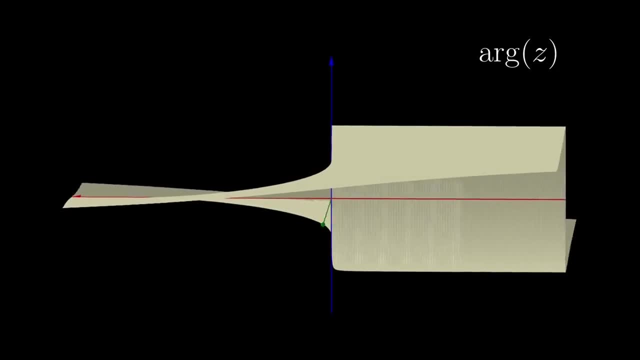 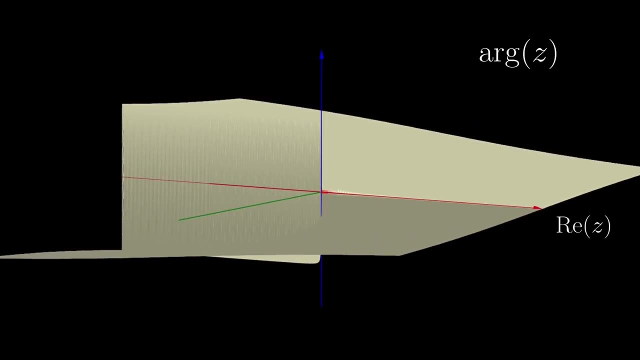 this is what we get. So we can see that on the positive real axis the argument is zero. As we go along the upper half plane, the argument increases up to positive pi. On the other hand, if we go to the lower half, 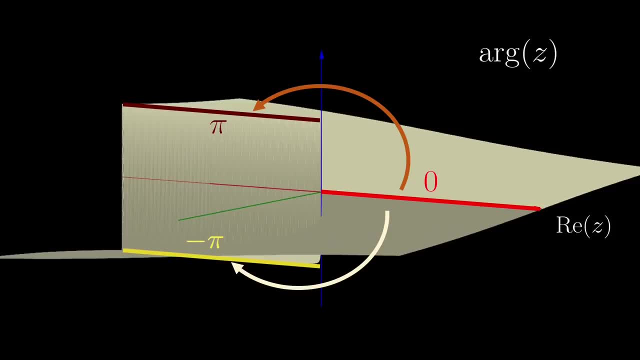 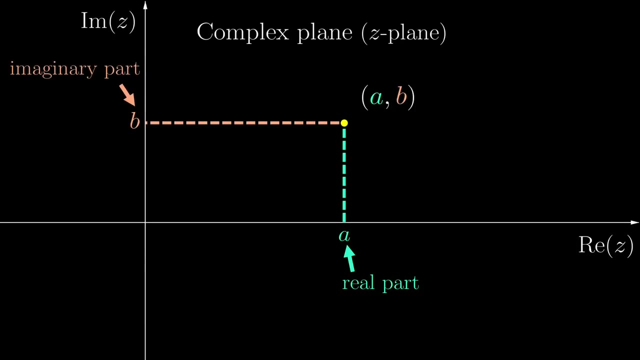 plane, the argument decreases to negative pi. You can see that there is a massive drop-off on the negative real axis, which is sometimes annoying. We will talk more about these problems in the next video. For now, let's go back to our normal complex plane. 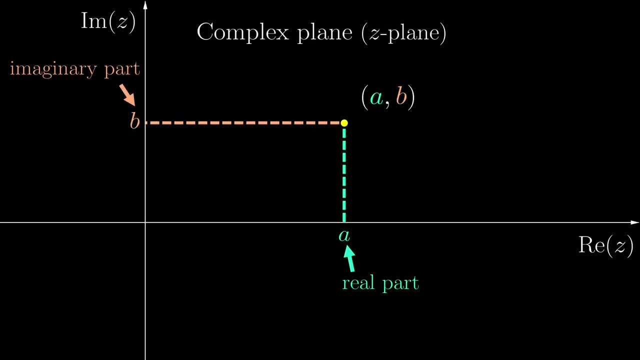 This is the Cartesian way of representing complex numbers and this is the polar way, Using simple trigonometry. on the right-angled triangle, it is not difficult to see that a is r cosine theta and b is r sine theta. So, apart from writing z as a plus bi, the other way is to use the. 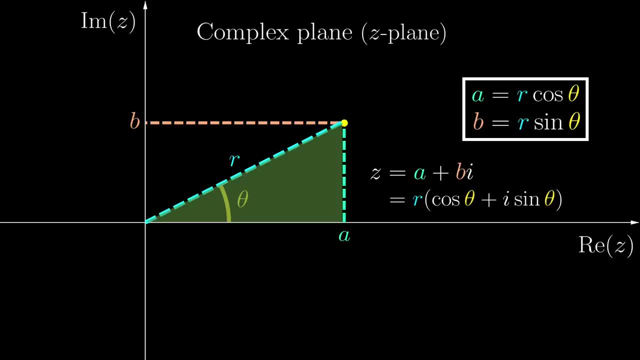 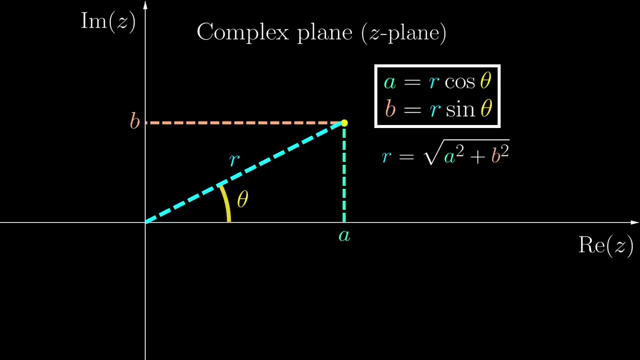 modulus and the argument. As we'll see later, this bit can be further simplified. Anyway, this white box represents how we know a and b from r and theta. but what about the other way around? Using Pythagorean theorem, r can be quite easily found, and if we focus on the 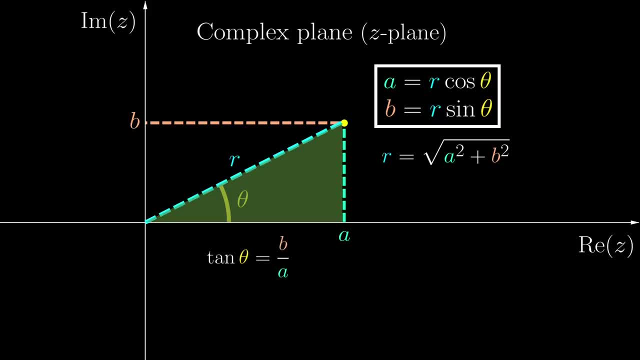 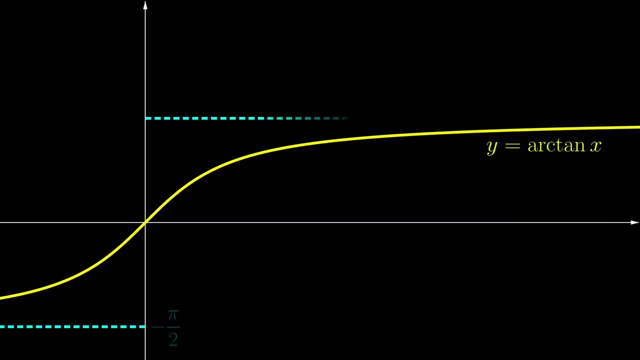 triangle, we can represent tangent theta as b over a, which seems to suggest that theta is arctan b over a, or is it? Remember that the argument is in the range negative pi- pi, but the arctangent function only ranges from negative pi over 2 to positive pi over 2, so clearly something's wrong. 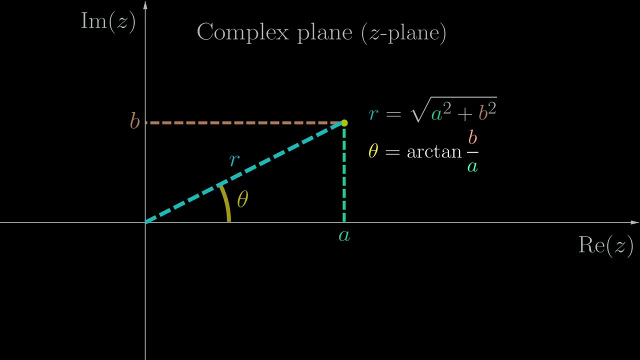 But this isn't completely wrong, though. If we are in the right-half plane, then this is perfectly fine, because in this case the range of theta matches exactly that of the arctangent function. But what's happening is that the ratio b over a 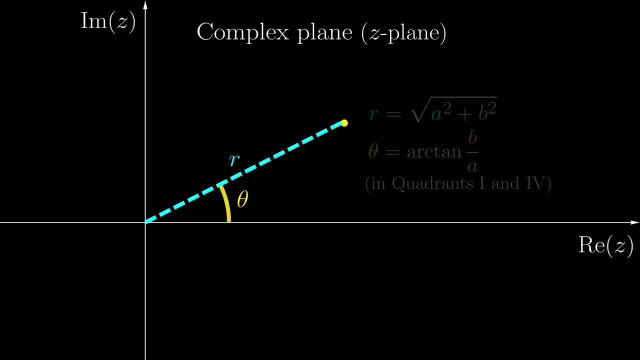 is the same on this line, but still the same even for points on the opposite side. But instead of having the positive argument, we would have a negative one, Since the arguments differ by pi, in this case it should be the arctangent minus pi. 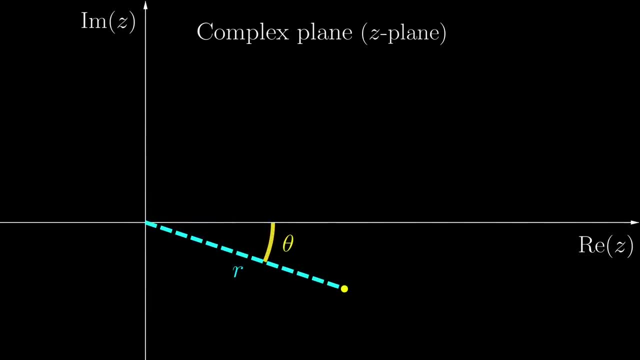 Similarly, the ratio b over a is unchanged, even on the other side of the line. and since this formula is perfectly fine in the fourth quadrant and the argument should have been positive rather than negative, in the second quadrant the argument should be the arctangent. 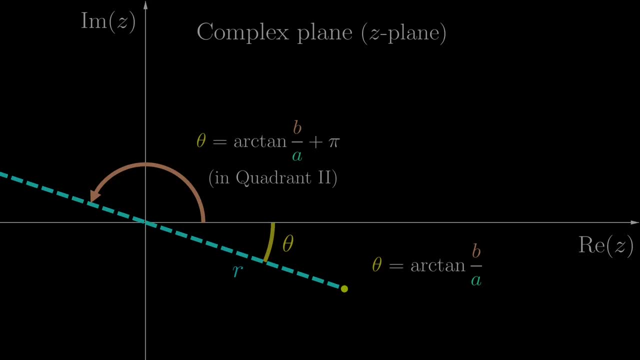 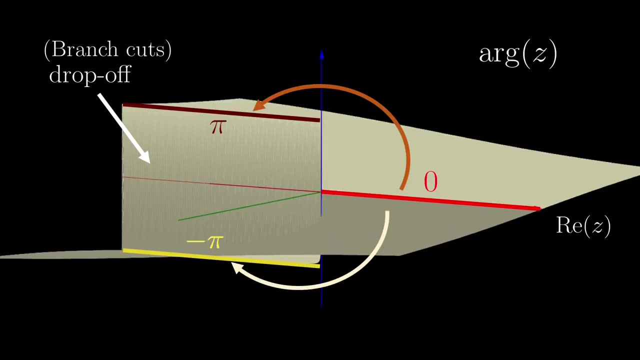 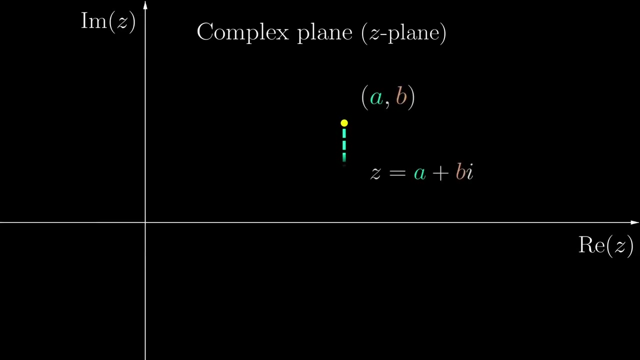 plus pi. Coupled with the issue of that massive drop-off, the argument function is not exactly the nicest function to work with, but we need to deal with it As a very quick recap. for any complex number we have the usual Cartesian way of representation. 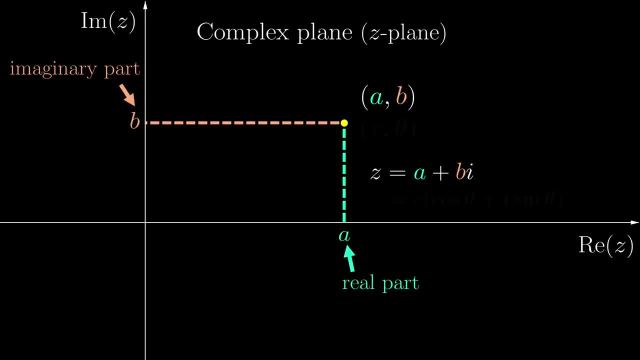 in terms of its real and imaginary parts, But also the polo way of representation using the modulus and the argument, And this box is the interconversion between the two ways of representation. However, one thing before we close this chapter: Instead of thinking about the complex number as a point, we can also think of it as a vector. 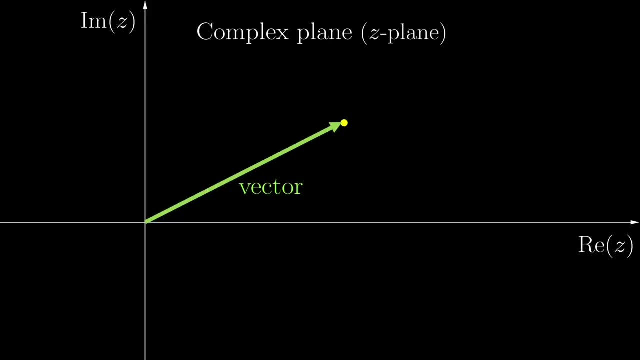 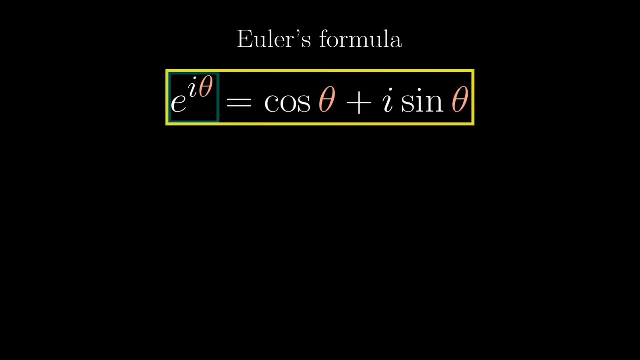 emanating from the origin. And now we move on. Euler's formula is the gateway to study more about complex numbers, But to actually derive it it depends on how you define the exponential function. There will be three proofs based on three definitions in this. 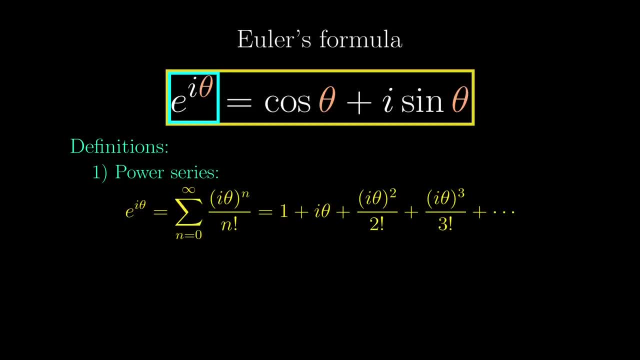 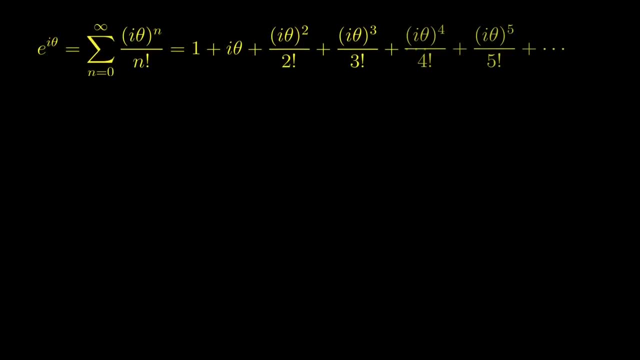 video, The most common definition would be the power series. If this is how you define exponentials, then you should be able to define the power series as the power series. This is the most classic way to prove the formula. We basically group every other term. 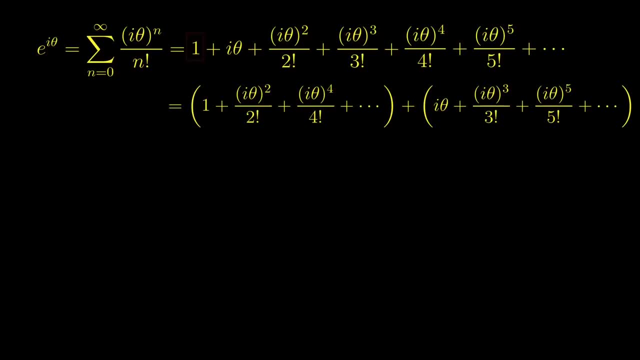 together And based on the definition that I squared equals negative 1,. we rewrite each bracket a little bit And now we recognize that the прокuh method outside of the souffle Regel记 된, all we just talked about. look, And the principal relation inside the suffle is the potential. 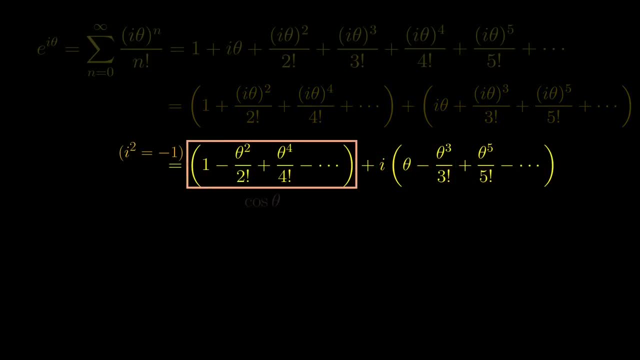 elephant. So root 1 for n. And well, I think- I won't specify the solution as two, because if I solved one I would get one, But if I solved one without a code- that the first series is that of cosine theta and the second series is sine theta, And so we 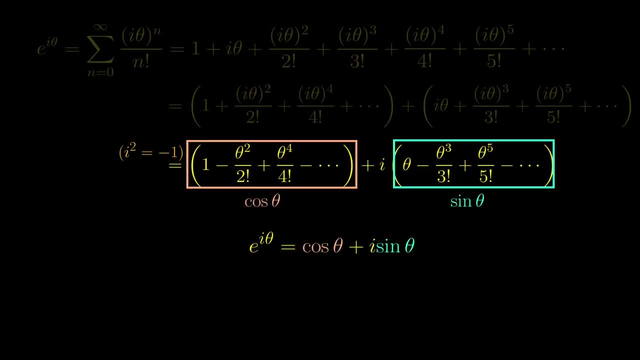 have e to the. i theta equals cosine theta plus i sine theta. But this proof isn't that illuminating, because why do these series correspond to sines and cosines? To address this problem, people usually simply define sines and cosines using these series, which well rigorously. 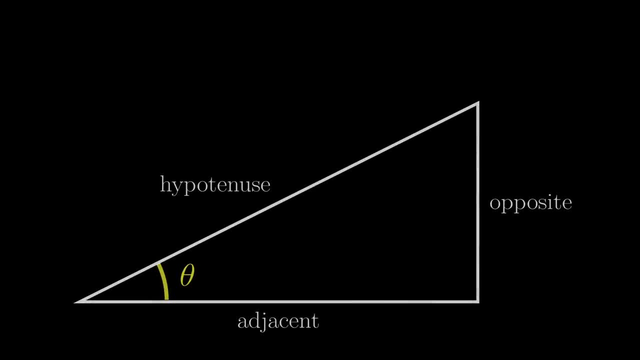 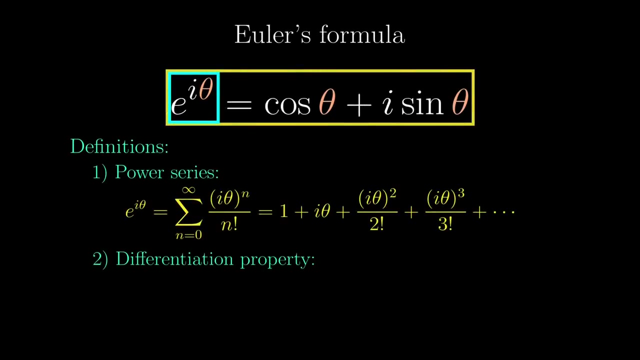 speaking isn't a problem, but how do these series even relate to the geometric characterizations of sines and cosines? It isn't impossible, but that's a story for another time. So we turn to the second definition of the exponential, which uses its property related. 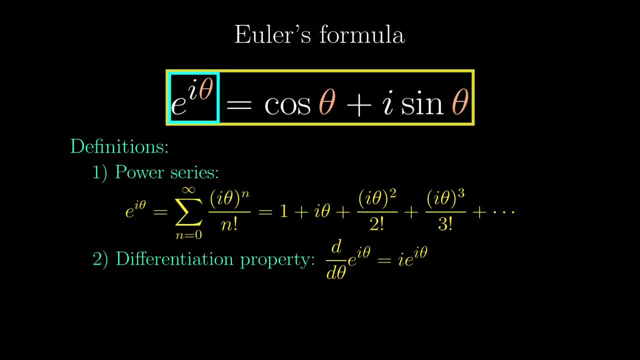 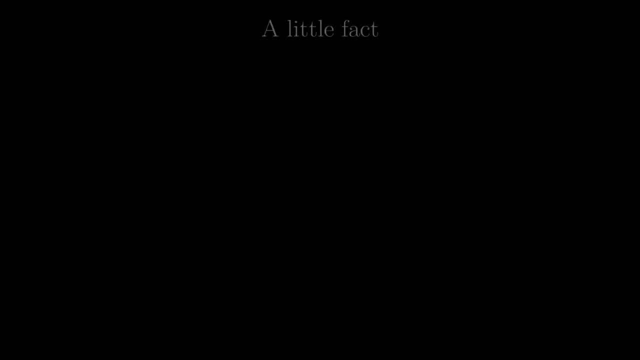 to differentiation, Namely, the derivative is simply i times itself, which is the basis of a nice visual proof. Before explaining this proof, we need a little bit of time. Final fact, which is how we multiply a complex number by i. When a is multiplied by i, 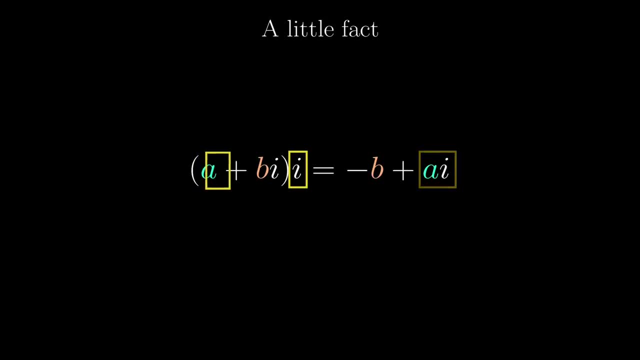 not too surprisingly, we get ai, And when bi is multiplied by i, we get negative b, because i squared equals negative 1.. This means that the point ab is mapped to the point negative ba by multiplication of i, But there is a really simple geometric illustration. This is the point. 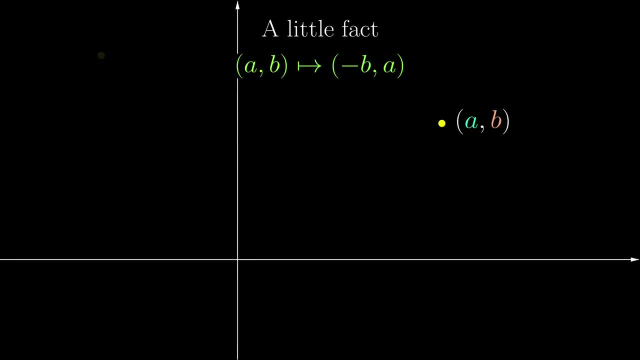 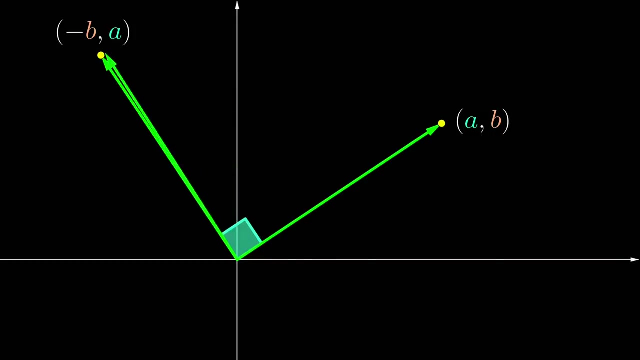 ab. After multiplying by i, we will get here negative ba. If we add the vectors and the angle, it might be a bit clearer what the multiplication by i does. Yes, it is simply a counterclockwise rotation about the origin by a right angle. And so we get onto the proof. 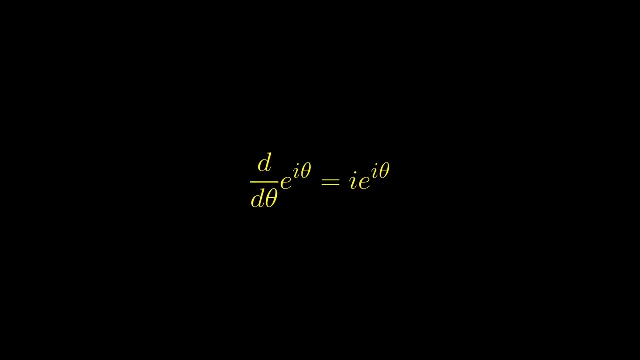 First of all, we need to understand what this derivative means. e to the i. theta can be thought of as your position on the complex plane, But the position changes with theta, so the changing positions create a trajectory. In this case, the trajectory isn't random. it is governed by this derivative equation, where 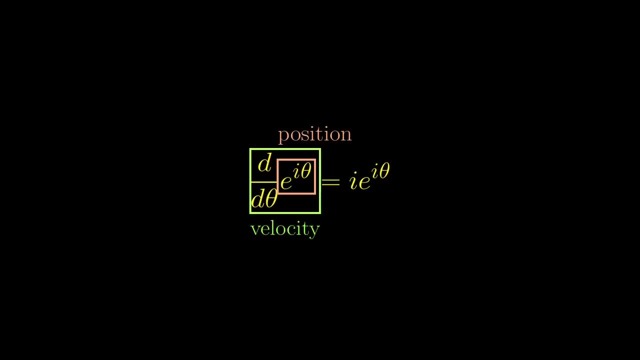 the left-hand side denotes the velocity of a particle following the trajectory. The right side is the position vector rotated anticlockwise about the origin by a right angle. This relation, together with the fact that when theta is zero, the expression of theta is zero, the 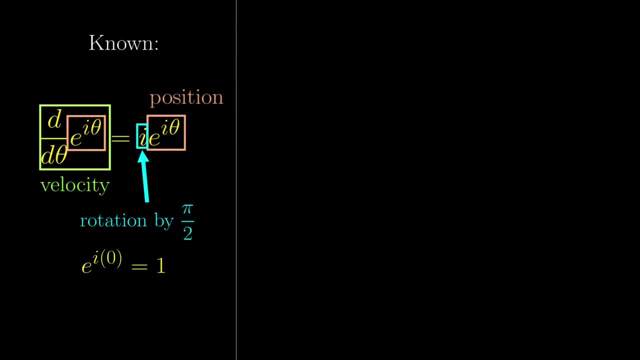 exponential is one allows us to determine the trajectory. So this is the complex plane. When theta is zero, it is one. so the particle starts here. Since the velocity is perpendicular to the position vector, the initial velocity points upwards. So after a very small time the velocity vector no longer points directly upwards. 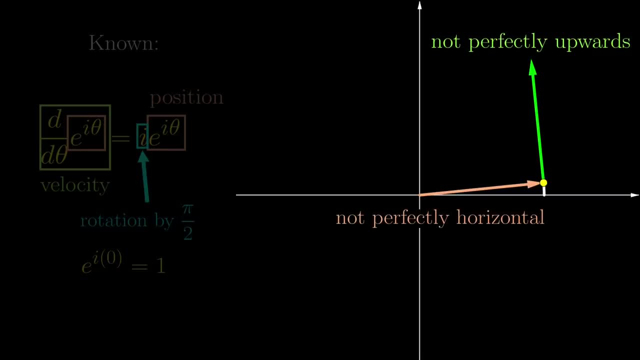 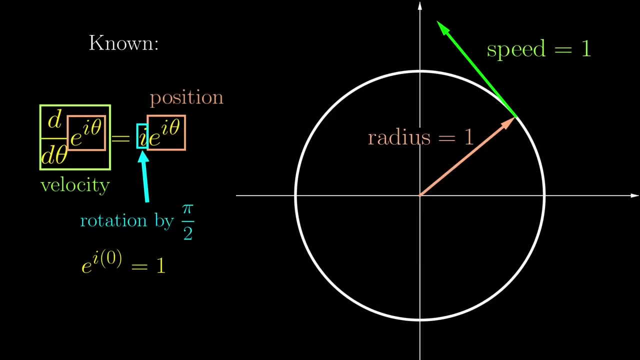 because the position vector is no longer perfectly horizontal. In fact, as time goes by, the trajectory is exactly a unit circle. Throughout the trajectory, the position vector has length 1, and so the speed is 1 throughout the journey, because the velocity is simply rotating. the 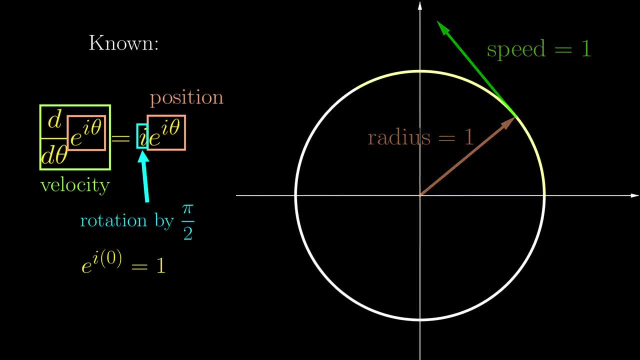 position vector with no stretching. So after time, theta, the distance travelled, is precisely theta, and so, by definition of angles in radian, the argument of this point is exactly theta. Because this point is equal to theta, the distance travelled is exactly theta, and so, 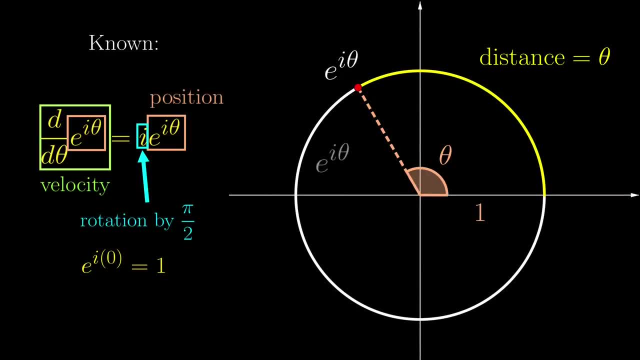 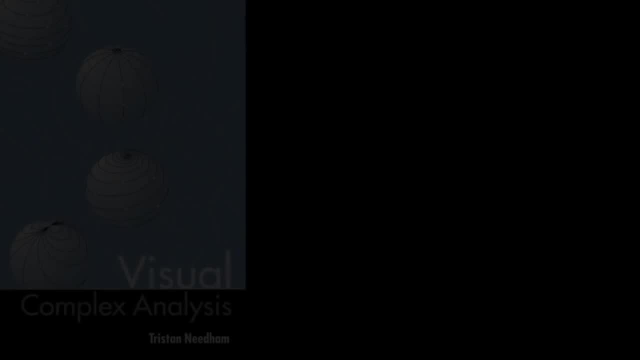 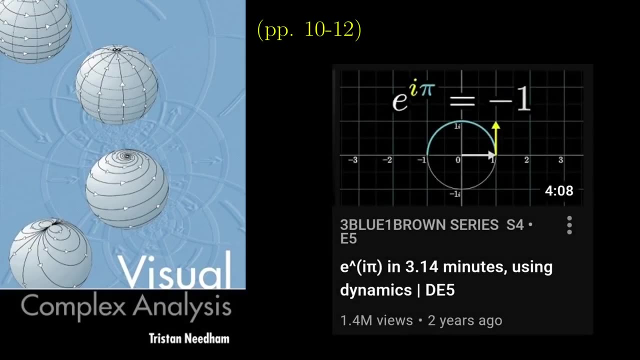 if we add e to the i theta, we finally get that e to the i. theta equals cosine theta plus i sine theta- Euler's formula. This amazing proof was, in visual complex analysis, mentioned in the previous video and also adapted by 3Blue1Brown in this video. So this proof uses the second definition of the. 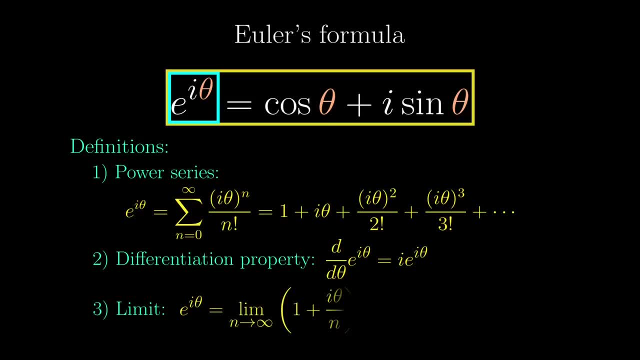 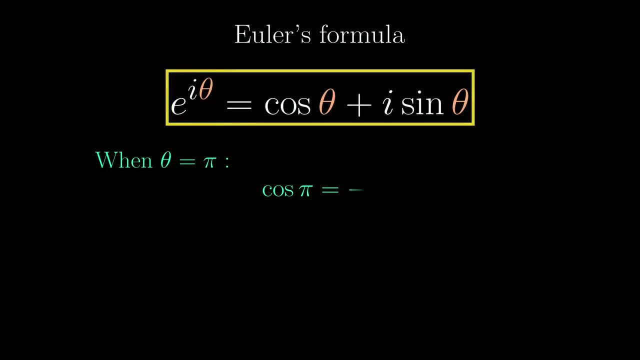 exponential. There is actually a third proof using the limit definition, but I'm going to put this off until later, where we'll get to that later. But let's consider the case where theta is pi, then cosine pi equals negative 1, and sine. 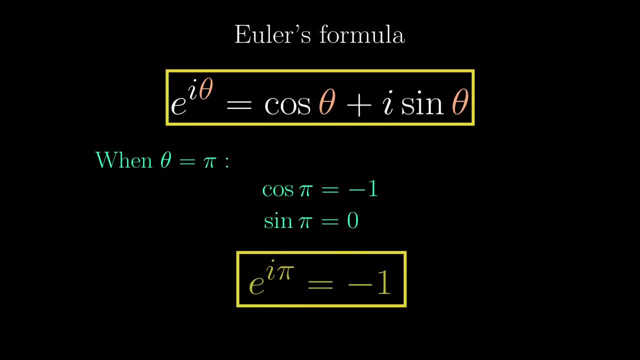 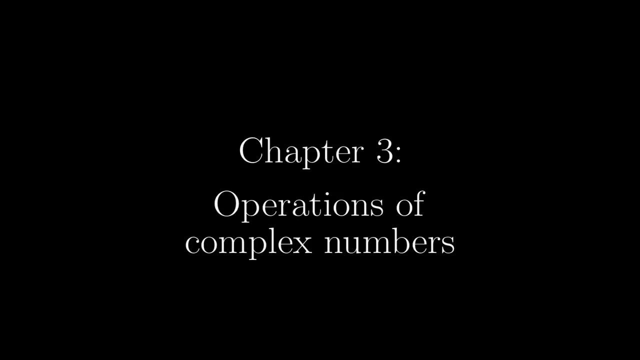 pi equals 0, and so e to the i pi equals negative 1.. This is usually called Euler's identity, which is often considered the most beautiful equation. How do we manipulate these complex numbers, then? Let's start with addition and subtraction, which is what you will expect. 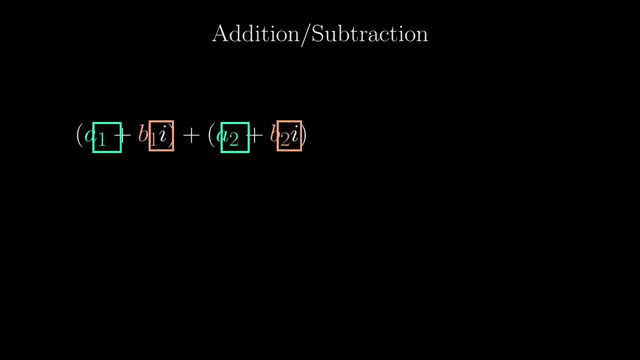 Adding two complex numbers simply means adding the real and imaginary parts separately. Similarly, subtracting two complex numbers means subtracting the real and imaginary parts separately. On the complex plane, adding two complex numbers is the same as adding two vectors together, so you either shift one of the vectors or apply the parallelogram rule to get the sign opposed. The real efforts, Hawaii, are the purely fundamental but also individual efforts, including the ounces of the square root of the total. So again, the real effort is in extra stress, so you should keep that coming. if you're not sure how to express it, butterfly, write all Odds. come on, Natalia, you better write it down. 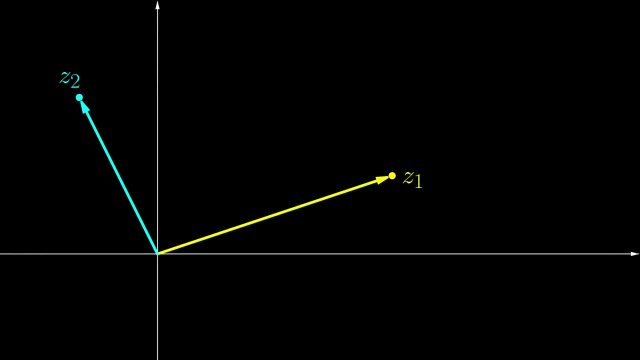 sum. If we are considering the difference, then this is simply the relative position of z1 from z2.. We simply translate so that it is emanating from the origin, and now z1 minus z2 is the tip of the vector. So addition and subtraction of complex numbers are rather 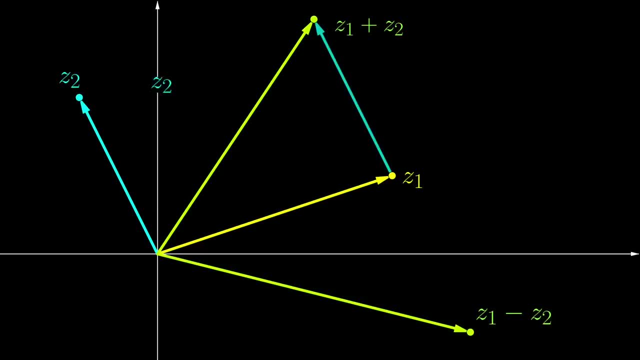 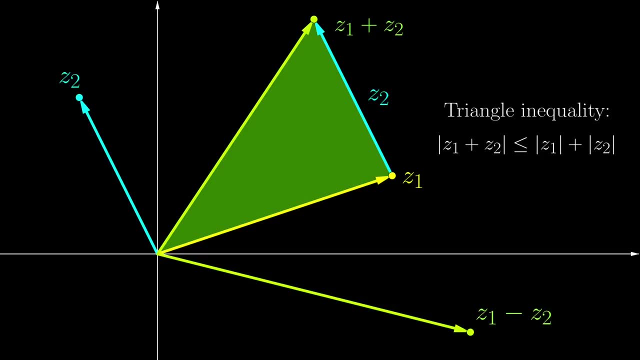 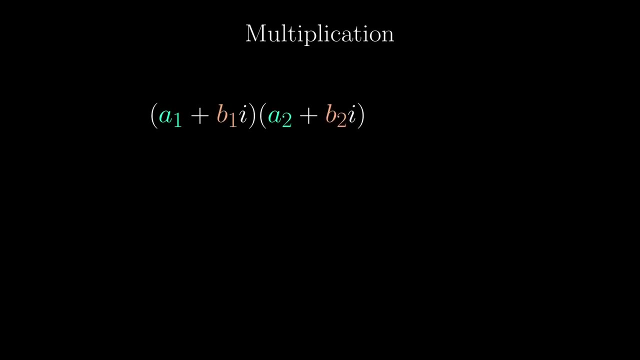 easy. Just one more thing. by normal triangle inequality on this triangle we get: the modulus of the sum is smaller than the sum of the moduli. And now let's get on to multiplication. To multiply two complex numbers expand, normally treating i as just another variable. but then 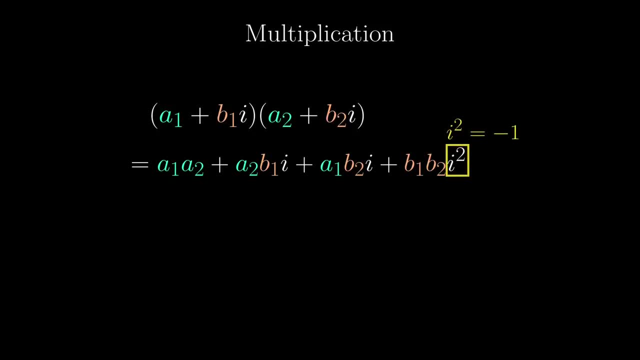 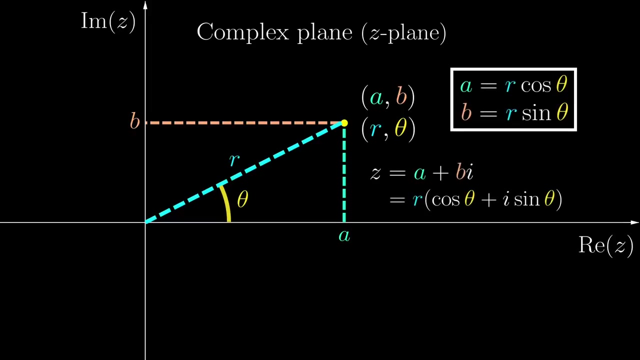 note that i squared equals negative 1, and separate the real and imaginary parts. This looks rather complicated. Is there a better way to do it? Remember that in the first chapter we have looked at the polar way of representing complex numbers. Now we know that the bracket is precisely e to the i theta because of the Euler's formula. 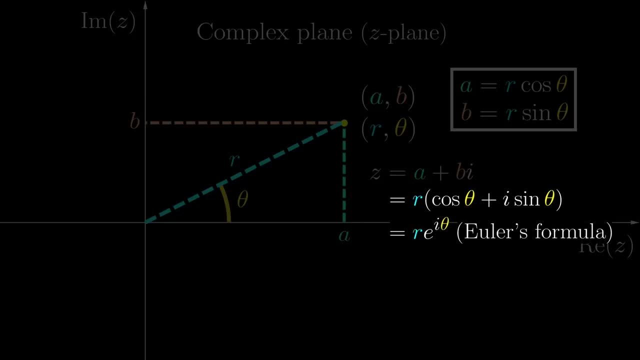 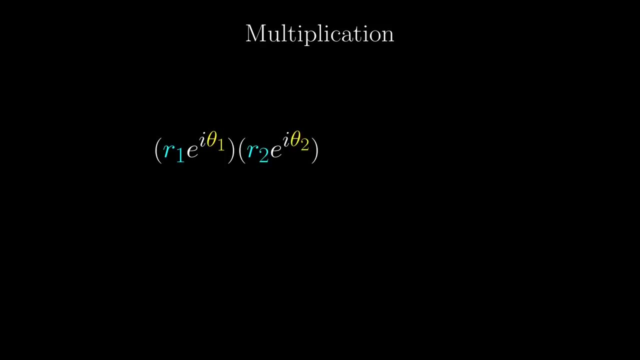 presented in the second chapter. So now, if we represent two complex numbers in this form, multiplication becomes a lot easier. The non-exponential parts multiply, and multiplying exponential particles become addition in the exponent. In other words, we multiply the moduli and 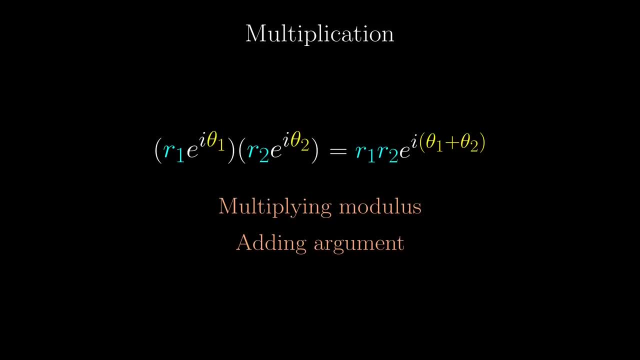 add the arguments together. Well, technically, not necessarily. THANK YOU, necessarily just adding, because while theta 1 and theta 2 are in the range for argument, it isn't necessarily the case that the sum is in the range. This equation is still true. 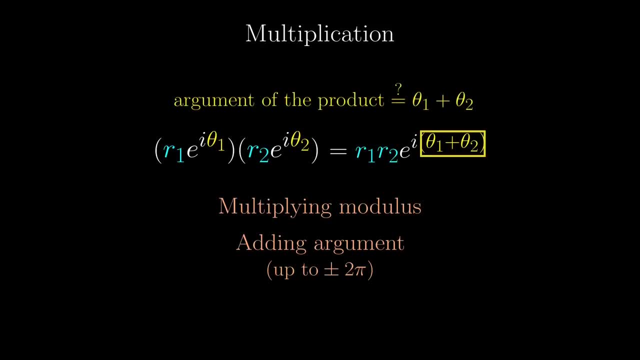 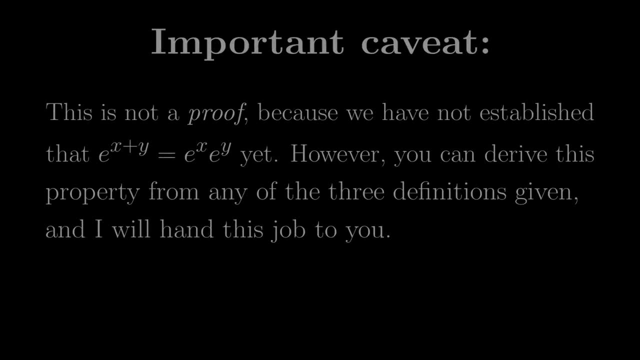 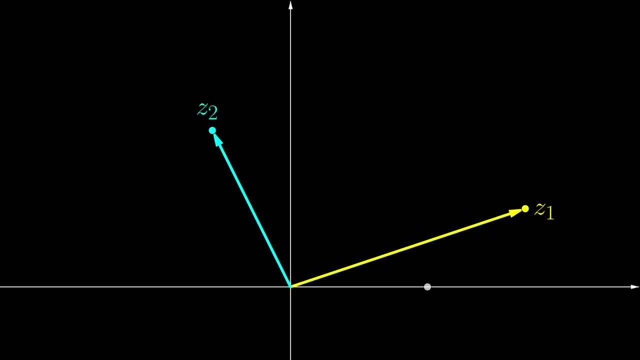 just that the thing inside the exponent is not necessarily the argument. The argument could differ from this by multiples of 2 pi On the complex plane. how do we multiply two complex numbers To do that? we identify where 1 is and construct a triangle with the origin 1 and z1 as the vertices. We then rotate the. 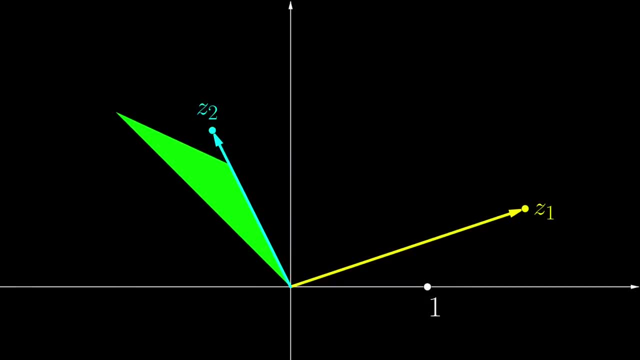 triangle so that the correct side aligns with z2, and then stretch it so that that side perfectly matches the vector representing z2, and the tip would represent the product. And I encourage you to think for yourself how this interpretation is related to the. 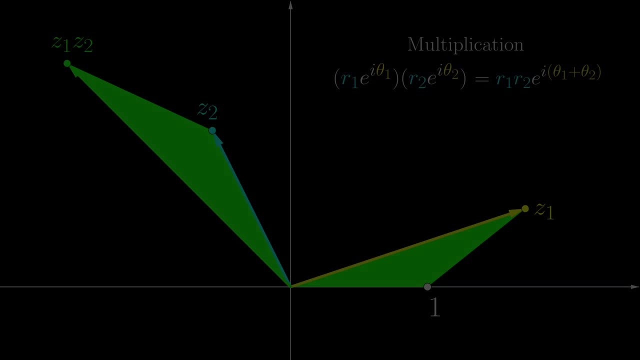 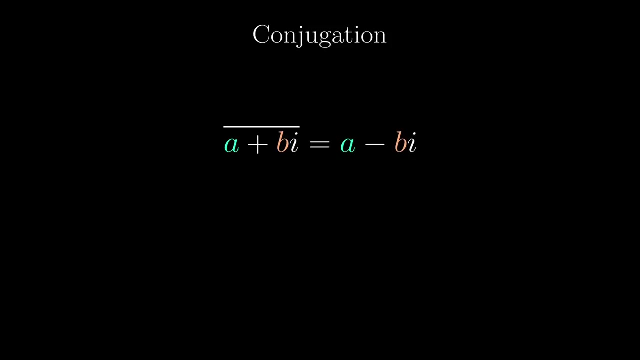 previous equation we have talked about And we now consider conjugation. The complex conjugate of any complex number is simply obtained by negating its imaginary part. In this video series, I'm going to use a bar of both to denote complex conjugation. 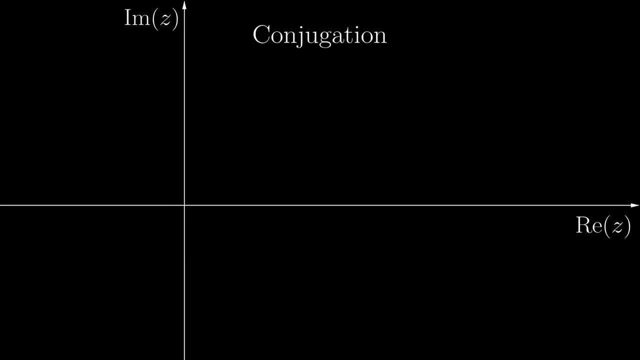 A geometric intuition is not too difficult to grasp either, For any complex number, z, its conjugate is simply its reflection across the real axis, which gives us another way of looking at it. Since we can always write z as z1,, we can also write z2 as z1.. 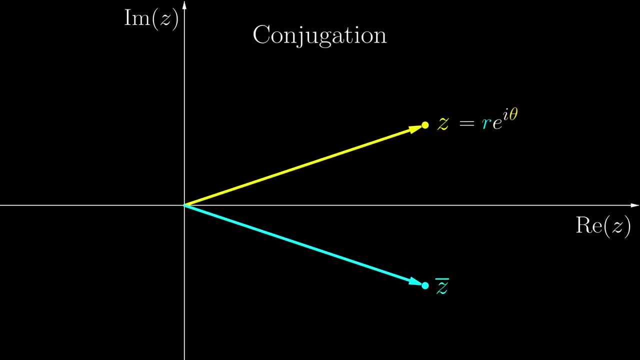 Since we can always write a complex number in terms of its modulus and argument, let's see what the corresponding information for z-bar might be. A simple reflection doesn't change the modulus, but the argument changes from positive to negative, and so z-bar is. 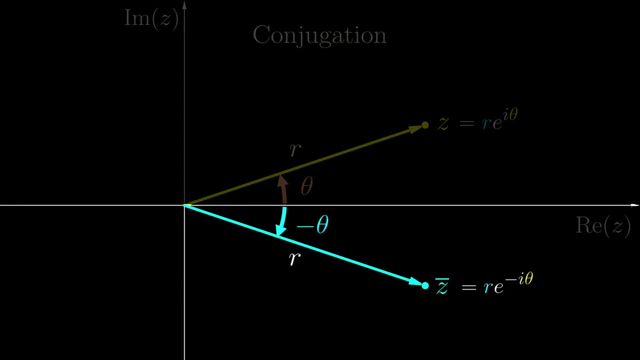 actually r? e to the negative i? theta. So this is another way of thinking about conjugation. With all these, let's consider the product of z and its conjugate. The algebraic way would be to first write z in its Cartesian form. Then the product can be rewritten. this: 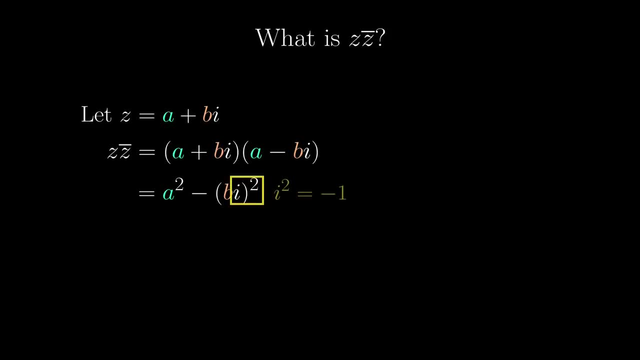 way and through some basic algebraic manipulations, we get that z is equal to a square plus b squared. But looking back at the form of z, it is simply the modulus squared, which simply came from applying the Pythagorean theorem. 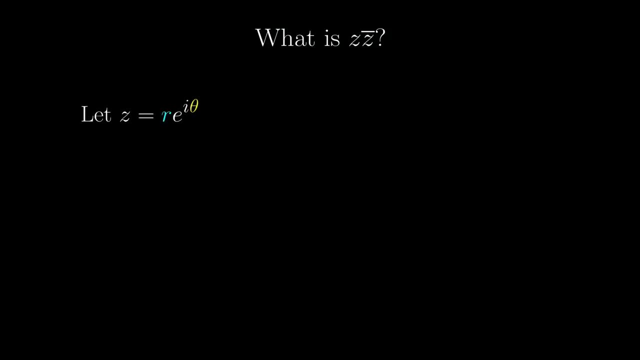 The other approach would be to write z in the polar form. then, from what we discussed, the conjugate has its argument negated. It can be written a way. the first way would be the first to write z in its Cartesian form. Then the product can be rewritten this way. 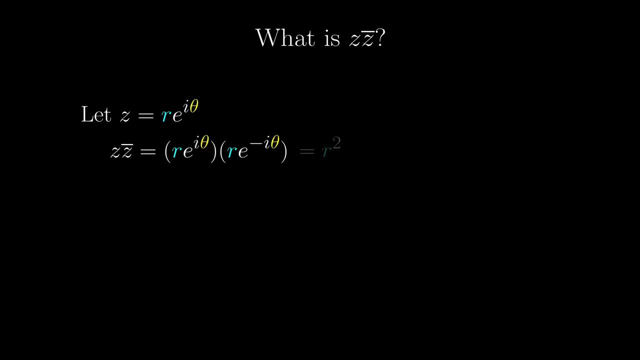 it and the exponentials cancel each other and we get again modulus squared. And this will be the inspiration for division of complex numbers. When it comes to division, the Cartesian form is quite messy. We first multiply both numerator and denominator by the same complex number, namely the conjugate of the original denominator. 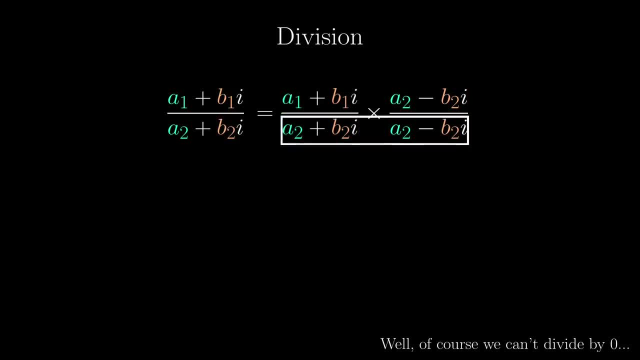 because now the denominator would be real, which is simply modulus squared. The numerator, however, is a mess, but this is only the product of two complex numbers which we knew how to deal with. To be honest, this expression is quite disgusting, but sometimes we do need. 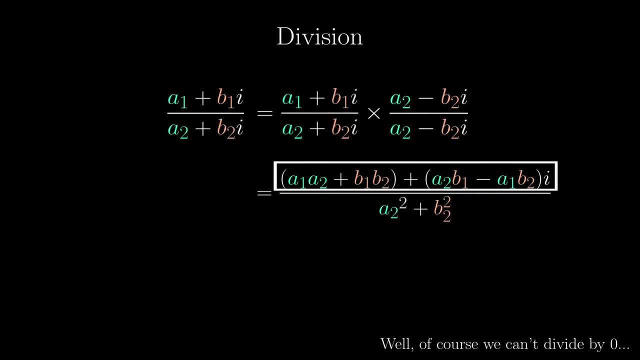 to know how to divide complex numbers this way. The much better way would be to write everything in polar form, quite similar to multiplication. that results in a very simple way. The result is rather nice. We divide the moduli and subtract the arguments. Well, 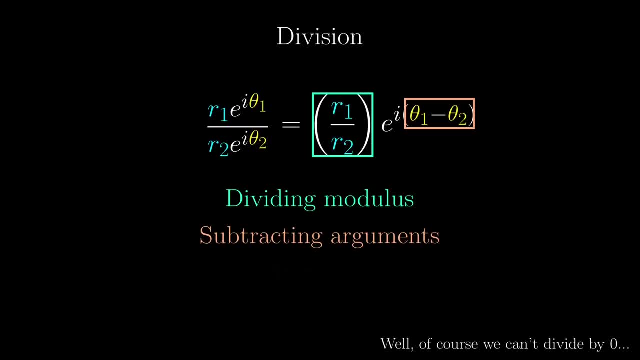 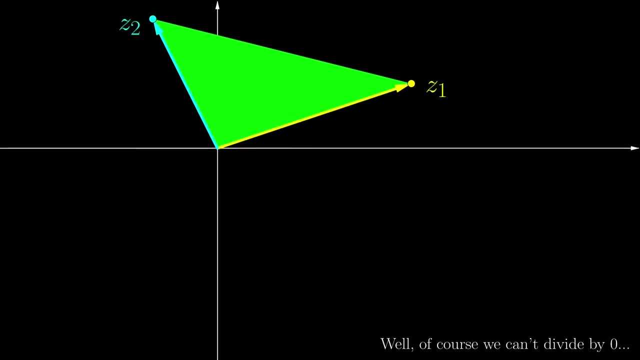 again, technically the argument isn't simply the difference. it could be different up to multiples of two pi On the complex plane. how do we divide two complex numbers? We first construct a triangle with z1,, z2, and the origin as vertices, then rotate it so that the side originally 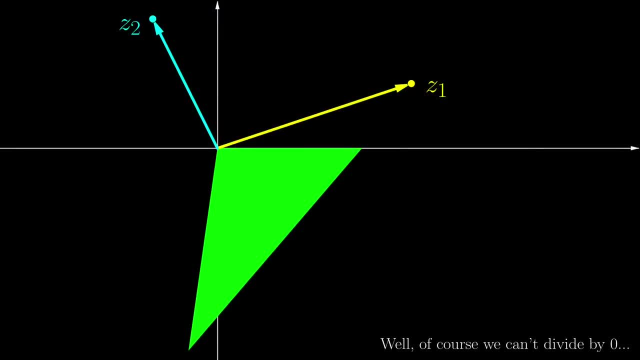 corresponding to z2 is aligned with the positive real axis. Then stretch, squish it so that the vertex on the real axis goes to 1, and then the tip would represent the quotient. Again, I encourage you to think about how this is related to the formula we. 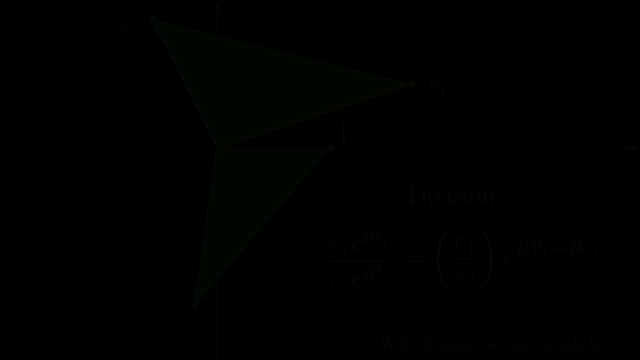 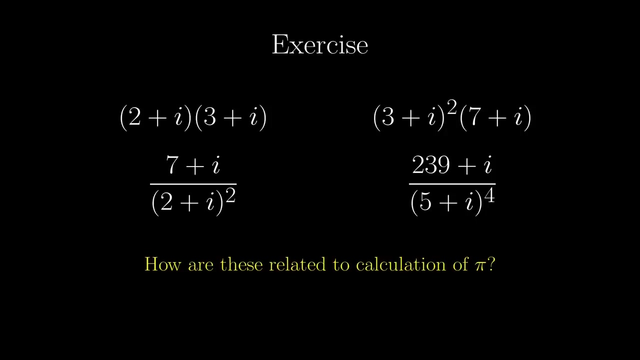 described earlier As a fun little exercise. consider these products or quotients and see how these are actually related to the calculation of pi. More details in this video. The final boss is a complex number to the power of another complex number To do that. 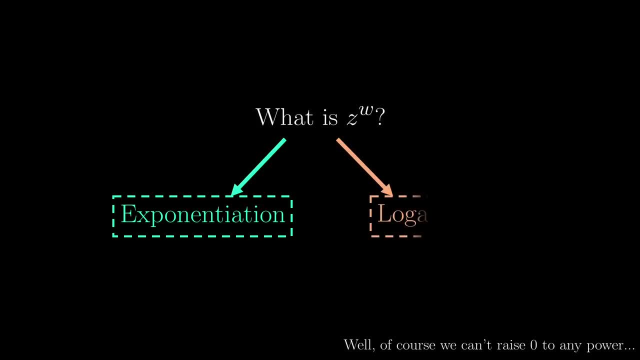 we need to know both exponentiation and logarithm. But let's tackle exponentiation first. Given z in its Cartesian form, what is the value of e to the z? Well, substitute normally into the expression and simply separate the real and imaginary parts, If you really want we. 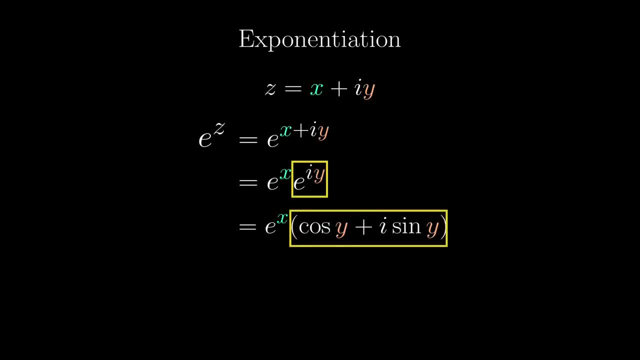 can further rewrite e to the i- y using Euler's formula. But let's focus on this second step. Isn't this similar to the polar form of a complex number? So the modulus is precisely e to the x. y is the argument? well, again, only up. 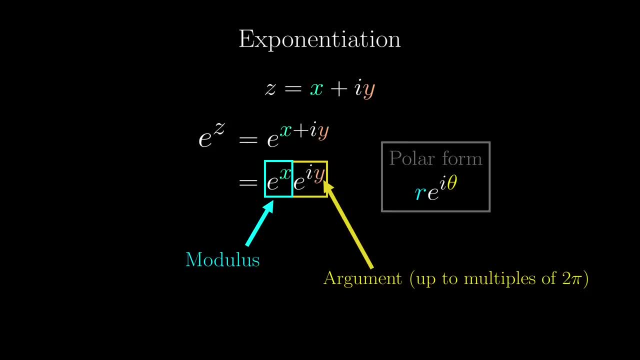 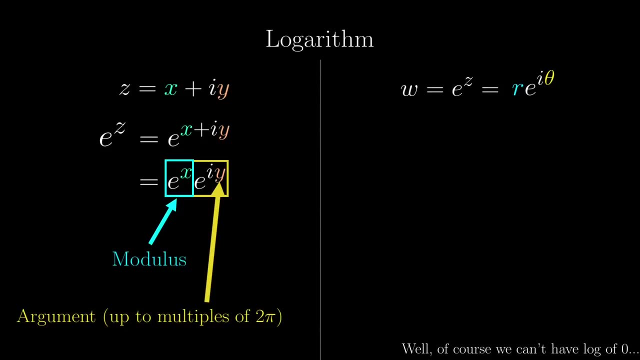 to multiples of 2 pi, And that could directly lead to how we define logarithms. If we have e to the z to be in polar form, how do we find out z? Well, just like what we said on the left, the modulus is e to the x, and so x is the usual logarithm. 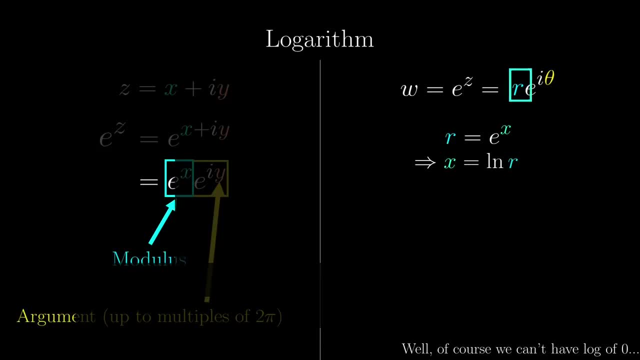 Real, natural logarithm of r. But what about y? As we saw just earlier, it should be the argument, right? Well, actually it could be the argument plus any multiple of 2 pi. So does this mean that the logarithm of w, which is z or x plus i, y, can take a lot of? 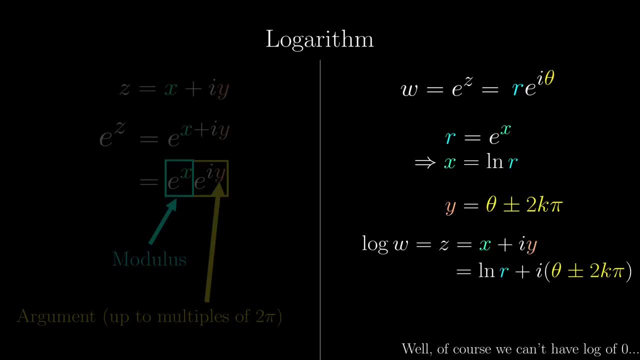 different values. Usually we only want one of the answers and we choose the one such that the imaginary part is in the range negative pi pi. So really it is just the argument of w. So with that, let's give a very simple example. 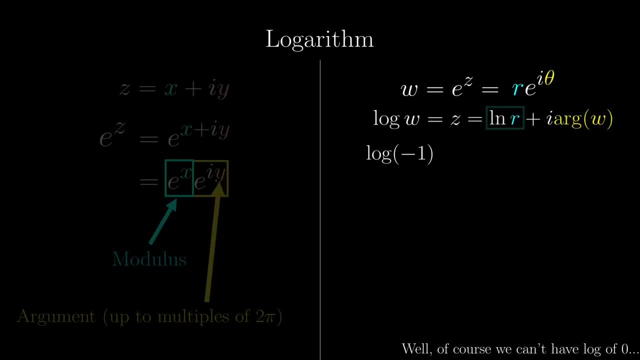 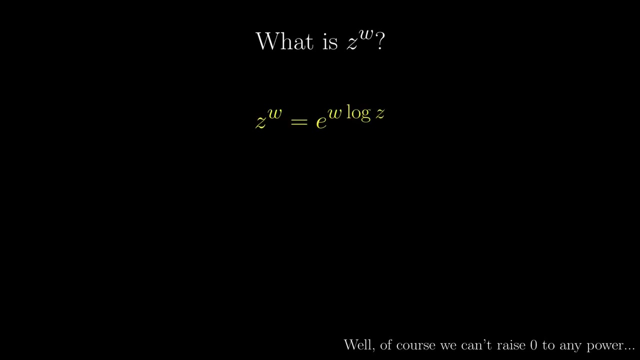 The logarithm of negative 1 is then the natural logarithm of its absolute value, 1 plus i times the argument, which is pi in this case, which means it is i, pi, And finally we see how we do complex exponents. This is completely analogous to the real case using both logarithm. 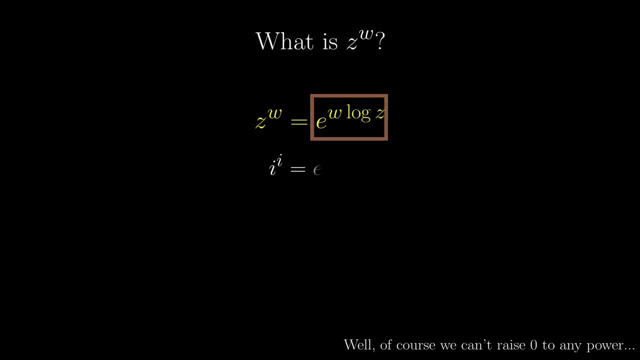 and exponentiation. To calculate i to the i we have to substitute z and w to be i in the definition and recall the logarithm of complex numbers explained just now. We can calculate the logarithm of i and after slight manipulation we get e to the negative pi over 2, a real number. 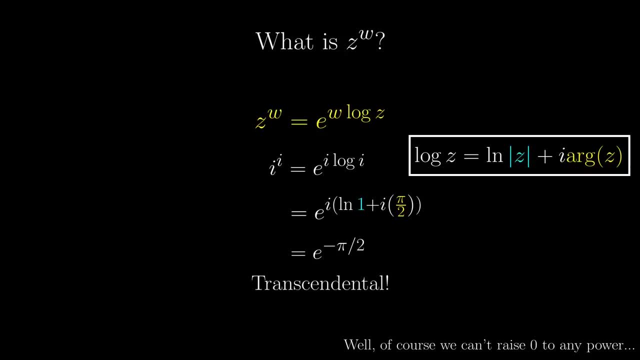 and transcendental as well. But before we wrap this chapter up, we need to revisit conjugation. Recall that if z equals a plus pi, i minus i plus i plus pi, then what is the real number? So we get z to the negative pi over 2, a real number and transcendental as well. But before we wrap this chapter up, we need to revisit conjugation. 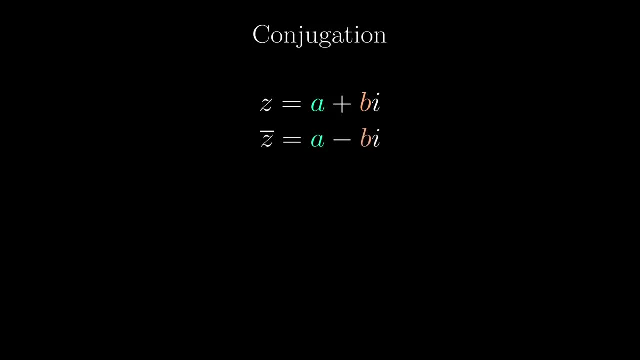 b i, then its conjugate is a minus b i. Let's say we now only know z and z bar. how do we find a and b, the real and imaginary parts of z? This is a relatively simple system of equations to solve, and you could and should verify these formulas A more geometric way. 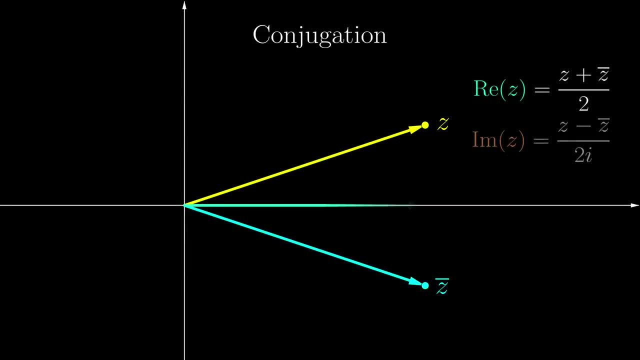 is to consider the complex plane. The real part is the average position of z and z bar, while the difference of z and z bar has length twice the imaginary part of z. But since the vector points vertically upwards, the difference is purely imaginary. so we have to divide. 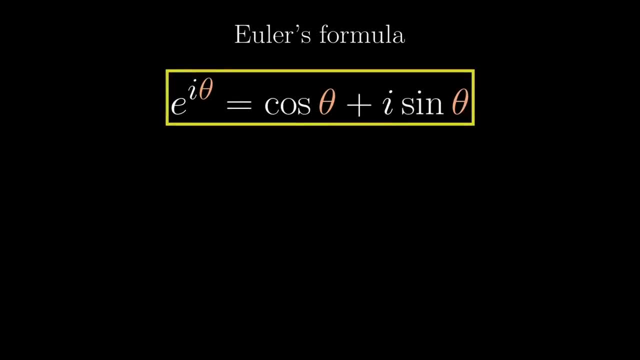 by i. Now let's get back to Euler's formula: Cosine theta is the real part, sine theta is the imaginary part, and since its conjugate is simply e to the negative, i theta. just like what we did a moment ago, we can write cosine. 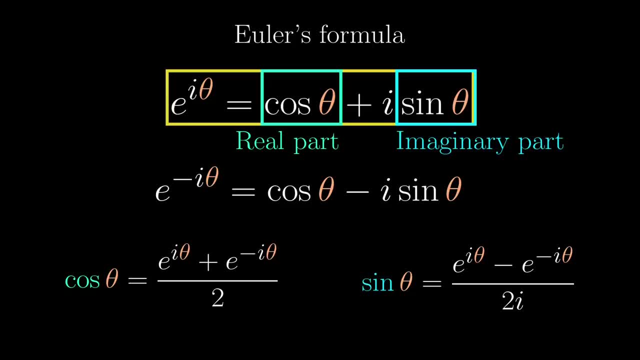 and sine as the imaginary part sine theta in terms of the exponentials. However, from the way we established it, this is only true when theta is real. so these formulas only make sense when theta is real. But we define cosine and sine of complex numbers using these formulas so that they remain true. 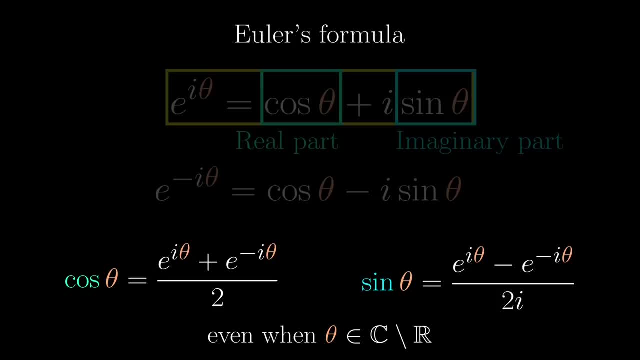 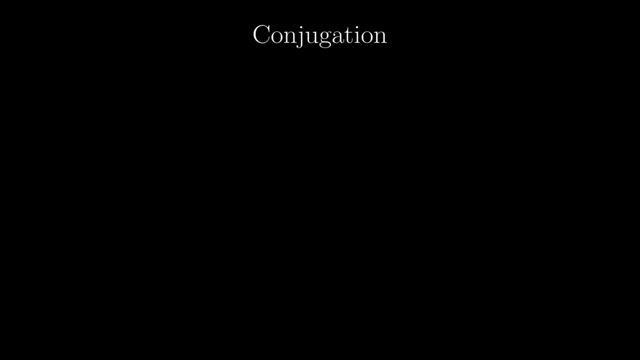 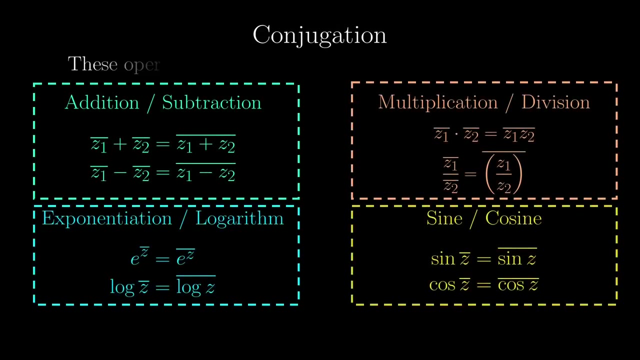 even when theta isn't real, Because now we know how to take e to any complex power. A final thing about conjugation, which is also a sort of summary of this chapter. Conjugation has all these properties, which looks a lot, but basically they say that the operations 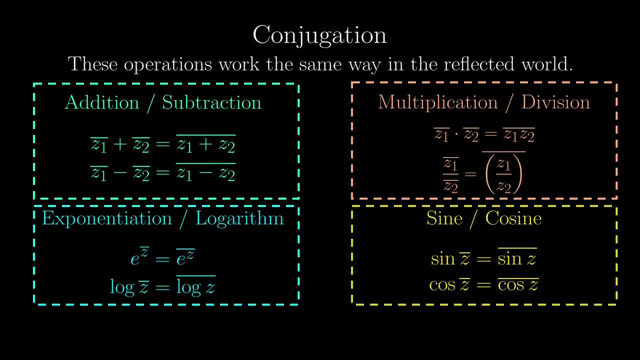 we have covered in this chapter work the same way in the reflected world, because conjugation is just reflecting in a real axis. And I do encourage you to verify all these properties of conjugation, not just algebraically but also geometrically, whenever you can, But in 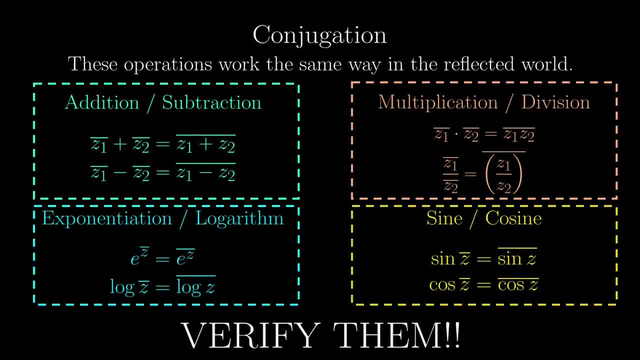 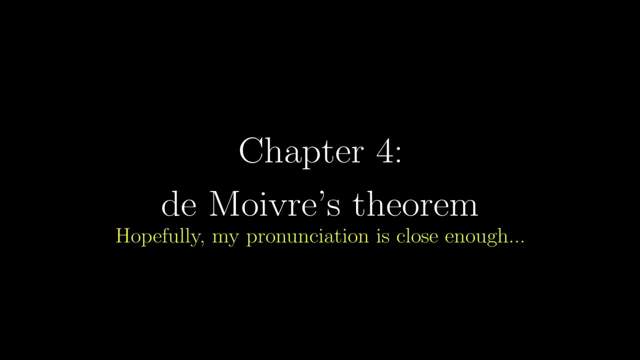 any case, these four types of operations are the major ones talked about in this long chapter. Previously we mentioned that if we multiply the complex numbers, we simply have to multiply the moduli and add up the arguments. So if we multiply n of them, we have a similar procedure. 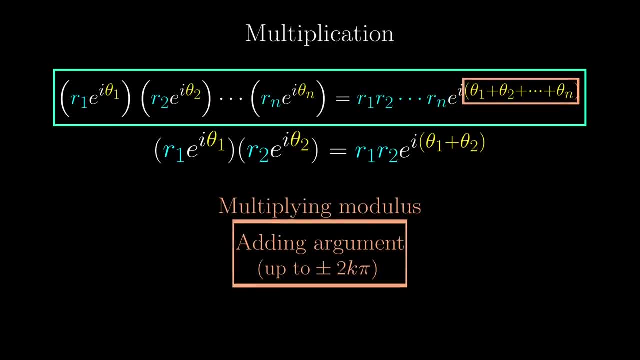 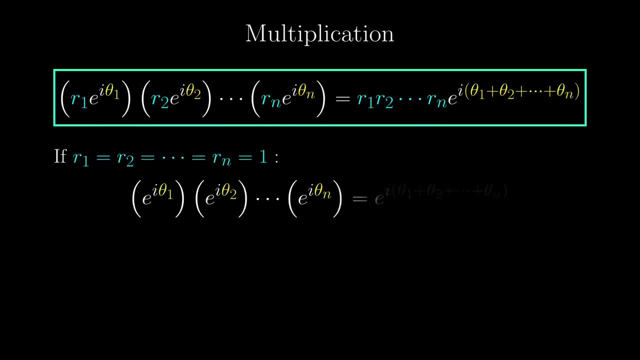 still multiplying the moduli and adding up the arguments. And so, in particular, if all the moduli are 1, that means that the arguments will be equal 1, then we only get the adding arguments bit. And if we further assume that all the arguments 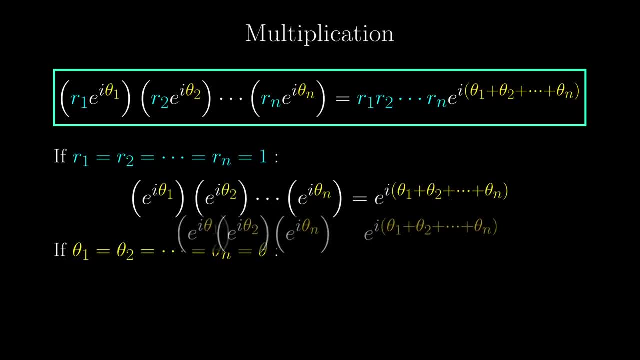 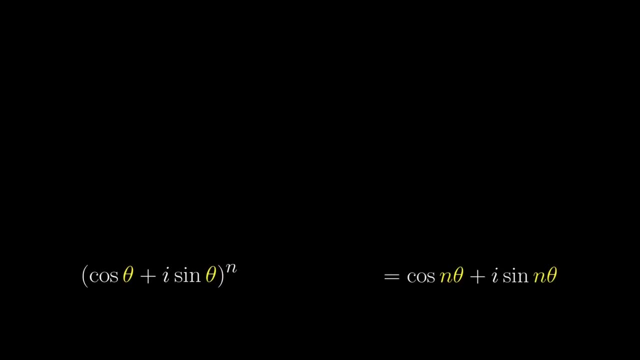 are the same being theta, then we get this. multiplying e to the i, theta by itself, n times is e to the i n theta. Using Euler's formula, we can rewrite the exponentials in the Cartesian form, and this is the Moivre's theorem. Note that n has to be an integer, but why dedicate? 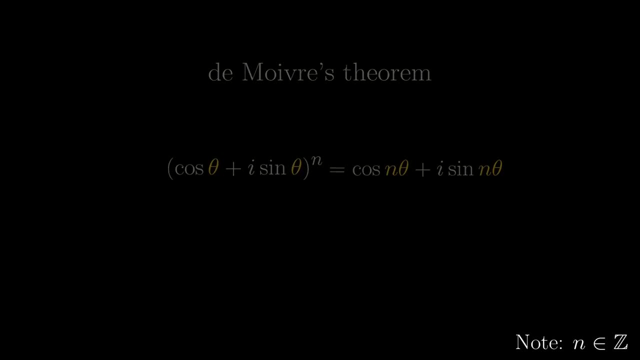 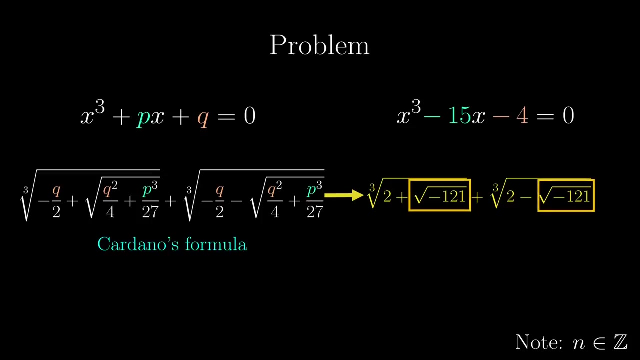 an entire chapter to this theorem. Remember that in the very beginning, the reason to start the study of complex numbers was the appearance of these square roots. but we also need to deal with the cube roots And the Moivre's theorem is going to be involved. 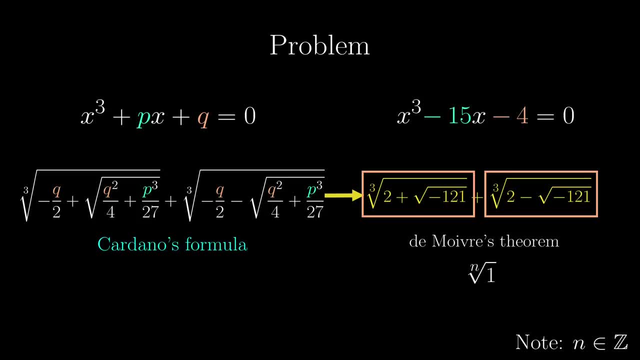 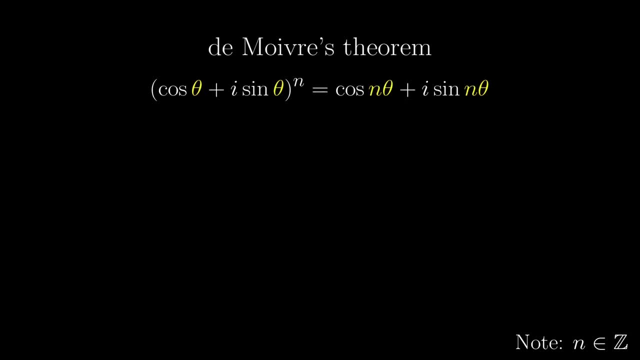 in finding cube roots, because it is generally useful in finding nth roots of one. Let's make the Moivre's theorem slightly more useful. We consider the nth power of a more general complex number. So we also have the modulus to consider. But the added modulus only changes the modulus. 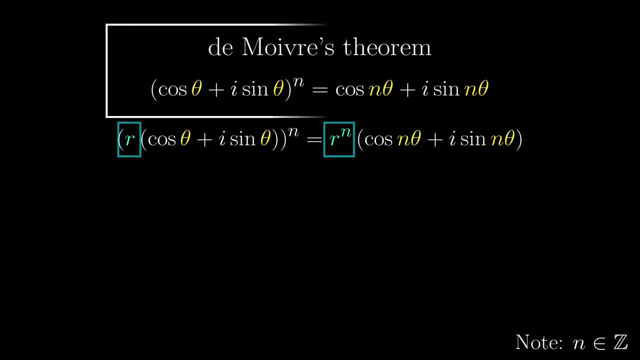 of the result to r to the n. Technically, the above is the De Moivre's theorem, but since the bottom one is just one step away, let's call the bottom one De Moivre's theorem from now on. The nth roots of one satisfy this equation by definition, and one could. 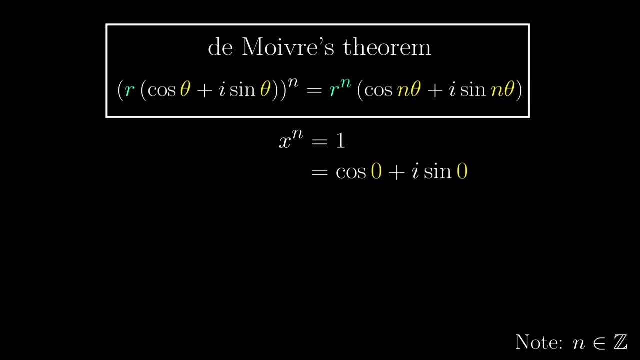 be represented in this polar form. Now compare it with the right hand side. Here the modulus is 1,, so r to the n is 1, and ntheta is 0.. For the first equation, r is the modulus, so it has to be real and positive. As long as n is not 0,, there's only one. 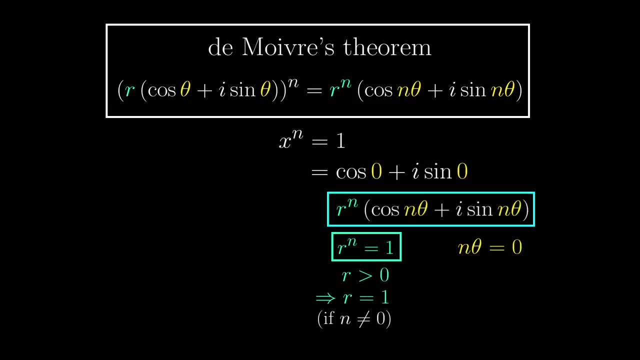 solution: r equals 1.. What about the other equation? Well, again, as long as n is not 0, theta can only be 0. Since, ultimately, x is r cosine theta plus i sine theta, by substituting values of r in theta, x equals 1, which definitely isn't surprising at all. However, that is. 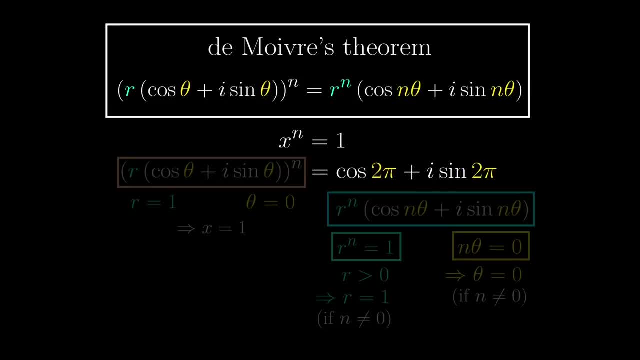 not the only way to write: 1. The angle could also have been 2 pi or 4 pi or 6 pi or, in general, 2k pi, where k is an integer. With these new representations, the first: 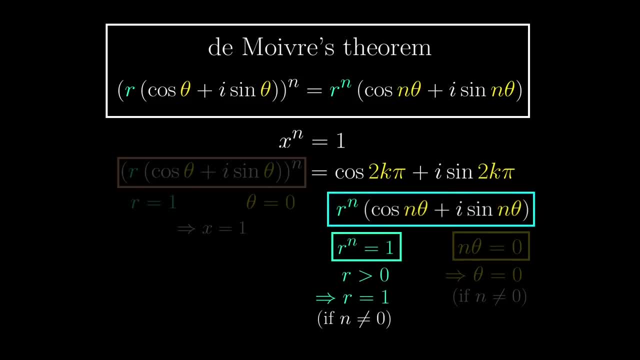 equation about the modulus wouldn't change, but the second equation would change, because now n theta is not just 0 anymore, but any multiple of 2 pi, and so theta is 2k pi over n, which means that the nth root can actually have a lot of different possible arguments. 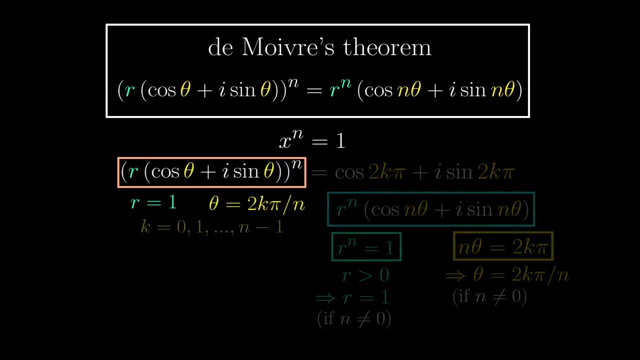 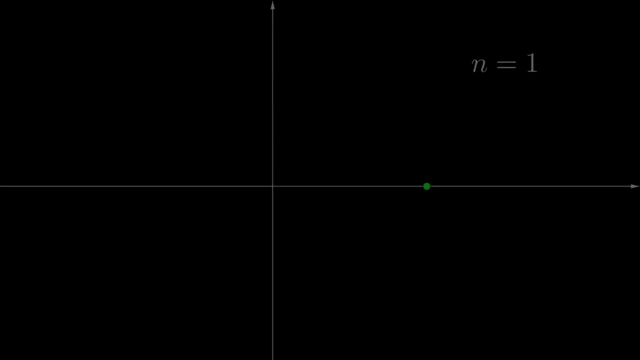 Well, actually exactly n of them, Namely from when k equals 0, all the way to n minus 1.. And these n different answers are called nth roots of unity. How do these roots of unity look on a complex plane? Well, when n equals 1, there is only one root, namely 1.. And when n gets large, 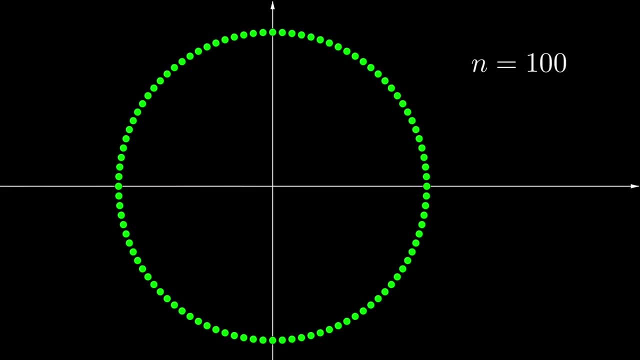 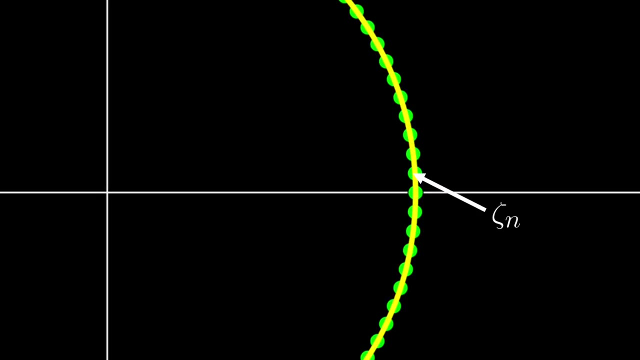 it is easier to see the pattern of these roots of unity. They all lie on the unit circle and are evenly spaced across the circumference. Usually the first one above 1 is important, denoted by zeta with subscript n, because now all of the other roots are powers of zeta n. 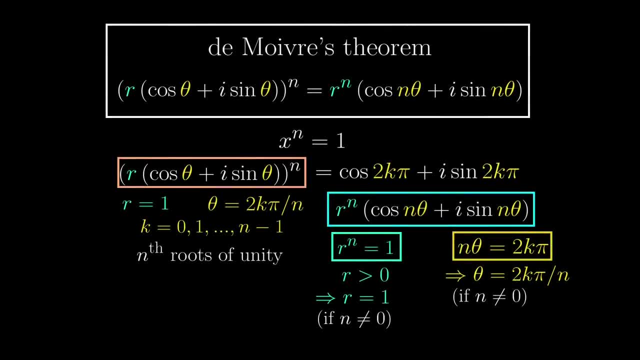 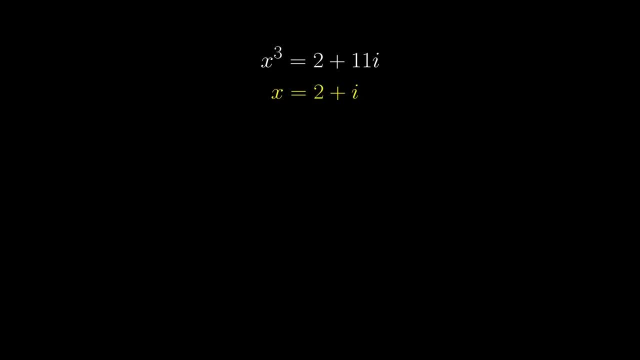 So, instead of using this procedure to find all nth roots, say, if we want to find cube roots of 2 plus 11i, we only need to find one of them, and then the others are obtained by multiplying powers of zeta 3.. Why, When we actually consider the solutions cubed, we then have 2 plus i. 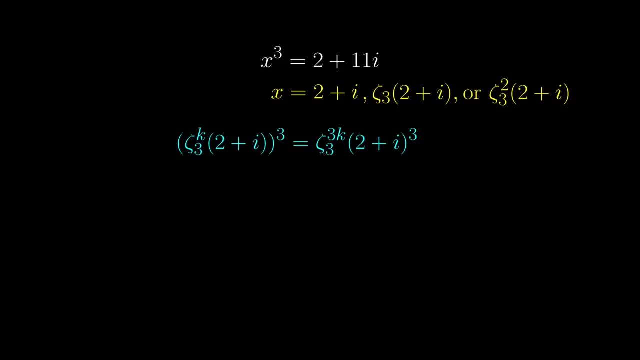 cubed with an additional factor. But by definition zeta 3 cubed is 1, so all these roots cubed to the same place. This means there are three cubed roots, but sometimes we have a preferred or a standard. 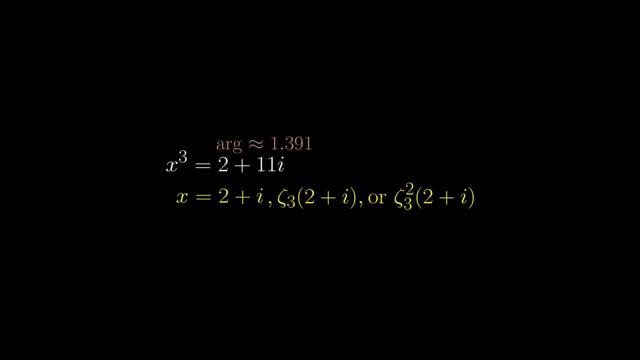 one. How do we choose? Well, we simply consider they're arguments. compared with the complex number we want to take, the cubed root of remembering that argument lives in the range negative pi pi. Then we choose the one with the argument: exactly a third of the original. In this case we choose 2 plus i with an argument exactly a third of the original. We then substitute as the next false loop that that happened and then use this step to throughout each Spieler representation. ay over, ay. Here we change the argument's numbers just like the first one, by a split of root and find that the numbers of N is or 28.. So 45 plus 38 plus 29.. And in the straights we find that it's 9.. So it's cos? OK, let's sum it up. Let's mid it down to 3 and start to solve the question. 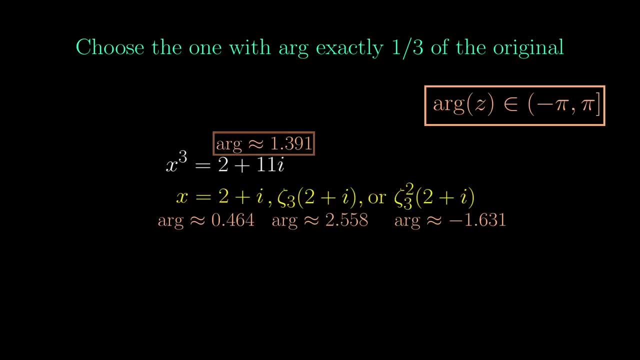 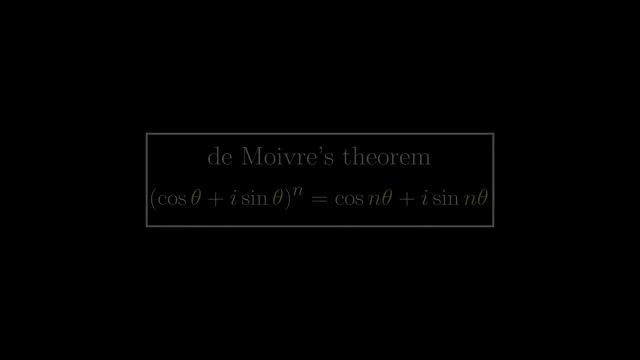 exactly a third of the original. and this choice using the arguments is called the principal cube root. And this is just one of the shenanigans of the Moivre's theorem. There is another, which is to prove Euler's formula. Wait what In this video we have literally. 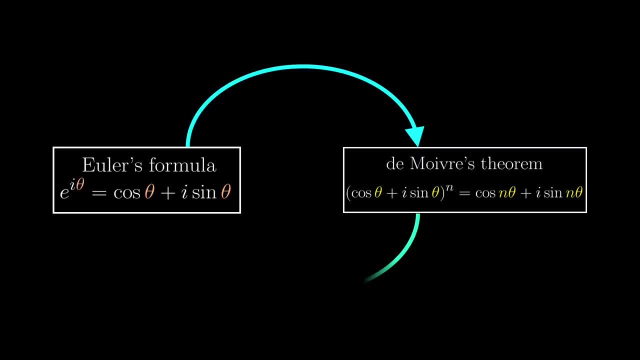 derived the Moivre's theorem from Euler's formula, and now you want to derive Euler's formula from the Moivre's theorem. This is a circle argument, But there is a way out if we didn't use the Euler's formula in the first place. In fact, it is possible. 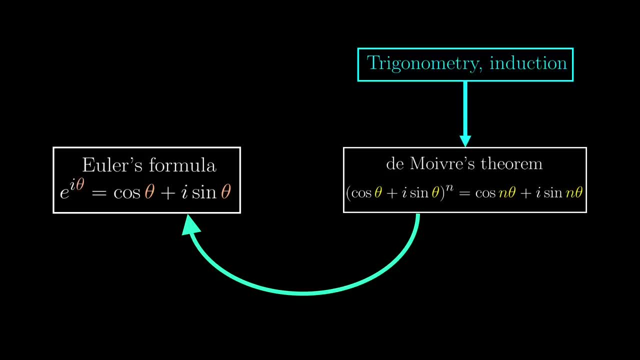 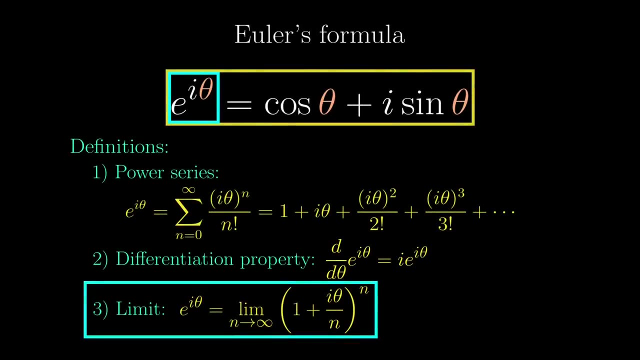 to only use compound angle formulas and induction, which does not rely on Euler's formula at all. so this is not really a circle argument. The bottom right to left implication is what the remainder of this video is about. The proof would start from the limit definition. 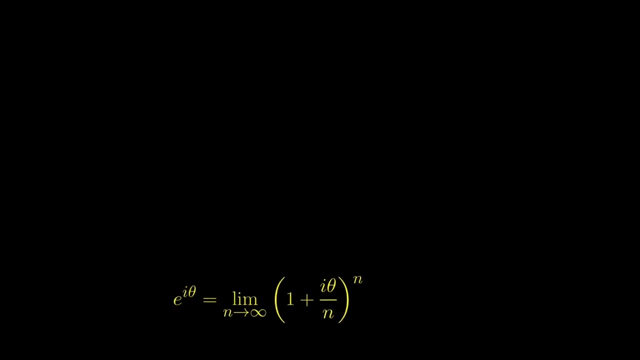 of the exponentials. Let's look at how this limit definition works visually. Let's look at how this limit definition works visually. First of all, we identify where 1 and 1 plus i theta over n are. We have chosen n to be. 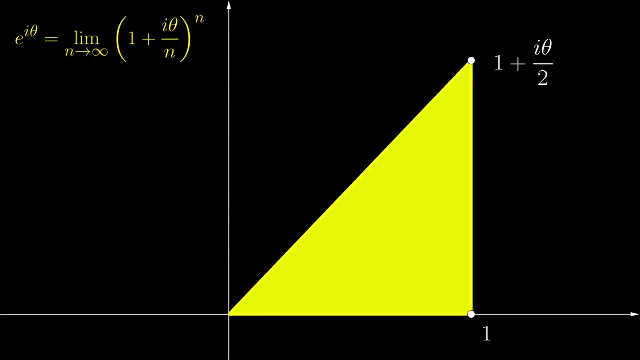 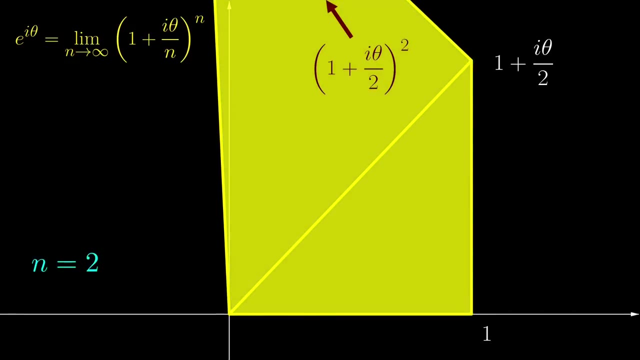 2 for now. We then construct a triangle with 0,, 1, and 1 plus i theta over 2 as vertices And, as we have illustrated before, rotate and stretch the triangle to get it square. But that is only the case when n equals 2.. We should increase the value of n and these 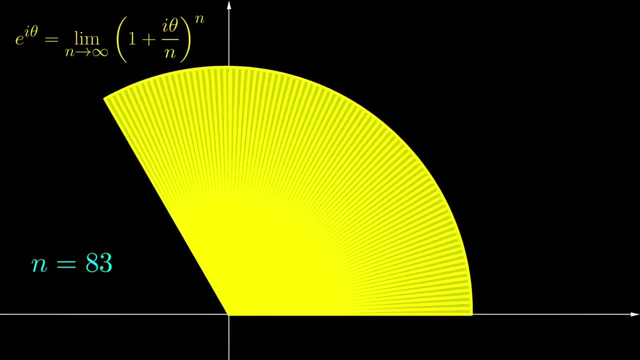 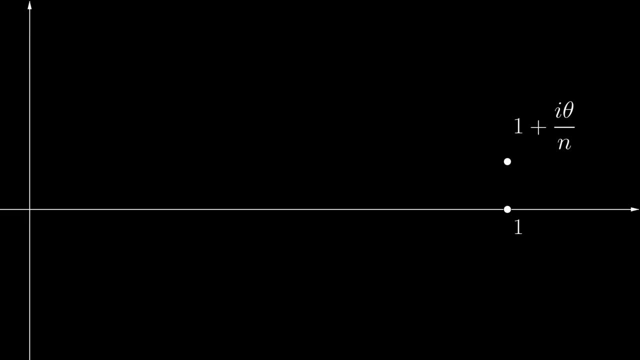 triangles together gradually become a zero. But how do we explain this phenomenon? Well, let's focus on a very tiny bit of the picture. before we draw the triangles, Let's add a part of the unit circle. While this point is not exactly on the unit circle, it will be closer and closer when n increases, Since 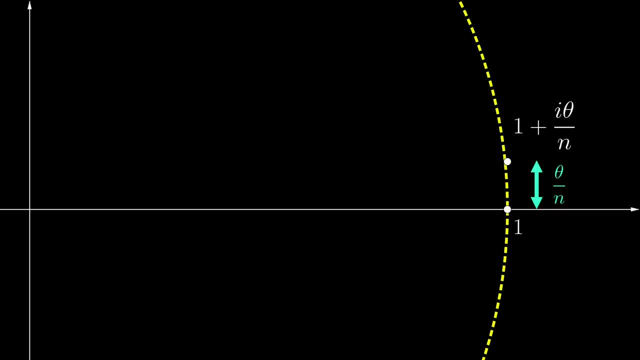 the distance here is theta over n. the angle subtended by definition of radians would also be theta over n. So we can see that the angle subtended would also be theta over n. So we can say that it is approximately cosine theta over n, plus i sine theta over n equal. 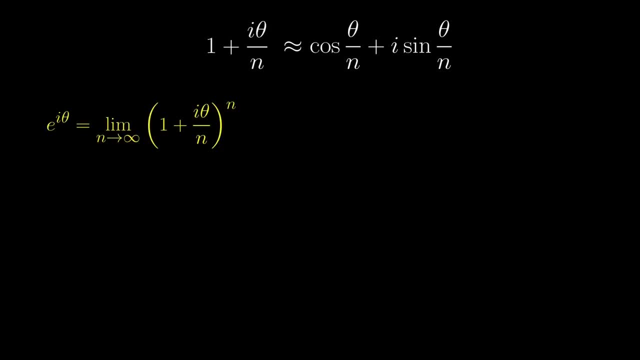 in the limit Now e to the i, theta being the limit of nth power of 1 plus i. theta over n can be rewritten like this By the Moivre theorem: the angle is multiplied by n, and so the limit is cosine theta plus i sine theta, Euler's formula. This proof was again in: 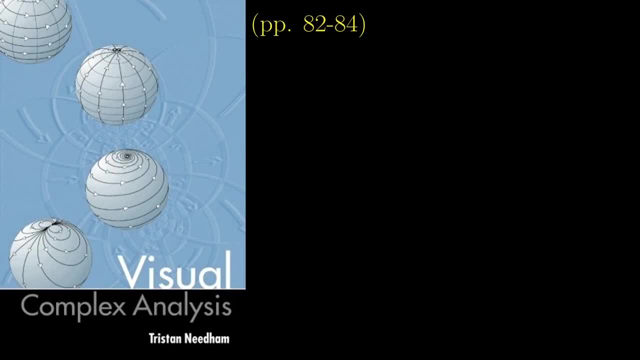 visual complex analysis mentioned earlier. So we can say that the angle subtended by definition of radians is the same as the angle of the area, But in fact the angle subtended here is less than or equal to the angle of the area.